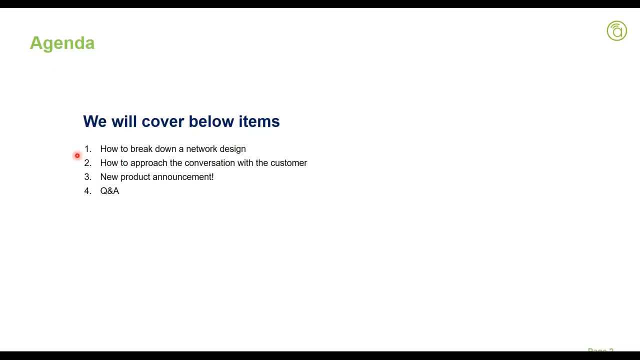 so you have a really good networking outcome. Okay, How can you have an opportunity with your customer? How can you design it? How can you think about that design to break down the solution in your head and come up with a really solid architecture. And second to that, you know what kind of conversation. 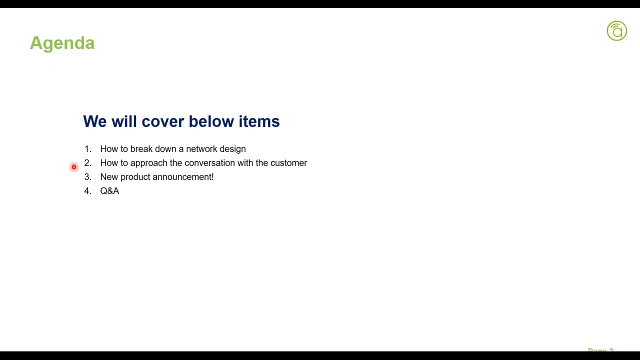 you need to have with your customer, What kind of input that you need to get from that customer in order to get to that really good approach. Before we end the presentation, we have some exciting and new product announcement for you, so stay tuned. for us, Something very 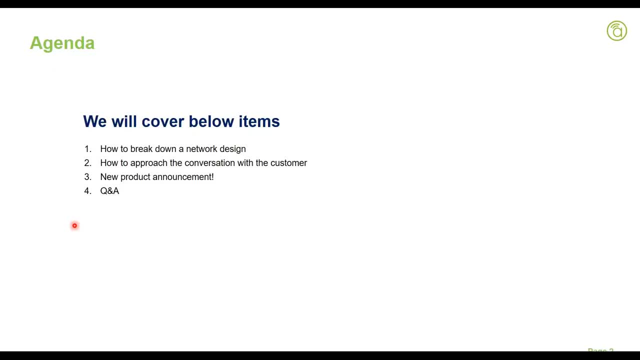 excited about and we'll end up with some Q&A. Thanks for a lot of your feedback. when you signed up for the webinar, I got to read all of the respondents' answers around. you know what kind of pain points you have today. I. 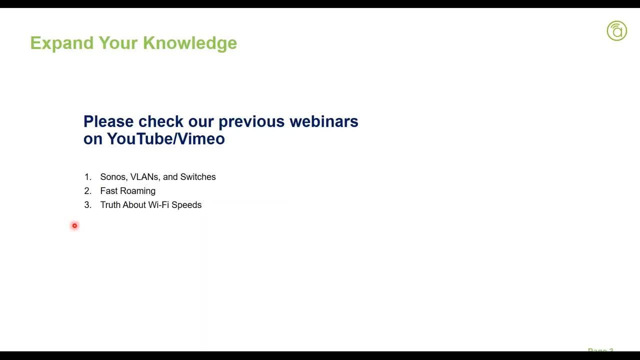 did see a lot of topics or pain points that we covered in previous webinars, so please check those webinar webinars, particularly those three. They are either on YouTube or Vimeo. So there's the Sonos, VLANs and switches webinar we did last year, So we talked about how to do VLAN setup. 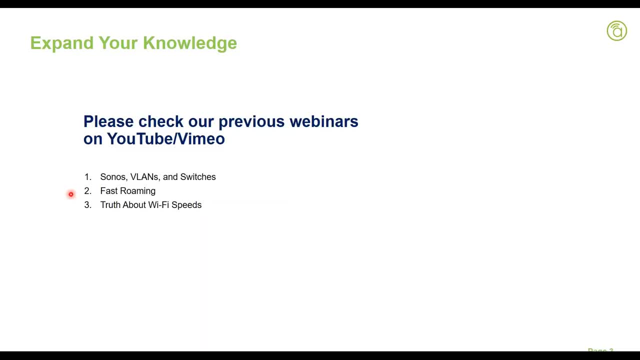 and deal with Sonos setups and all that fun stuff. And then we did fast roaming when we announced the 500, 700 access points, explaining how we deal with fast roaming on the access points themselves. And I believe last month we did the truth about Wi-Fi speeds, just to. 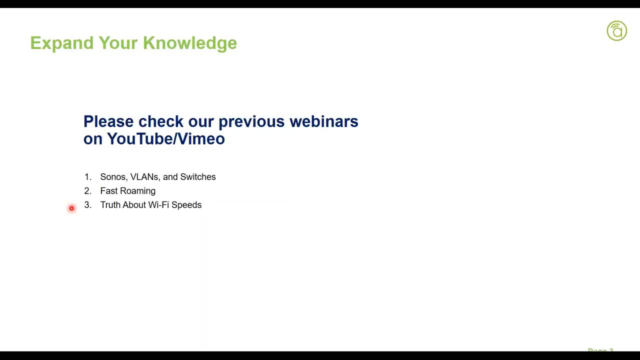 level set on what you should expect in the real world in terms of Wi-Fi speeds and how to level set that conversation with your customers. So today I will not dive into the details of each one of these three items. I'll leave it for you guys to go and kind of re-watch those webinars. 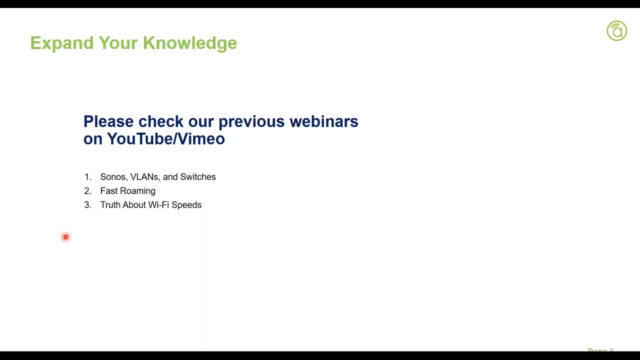 and brush up on that information, And we have a lot of time. We have a lot of content online in the product support tab as well. So, like I said, today is all about the architecture. So how can you design a new networking job? How can you? 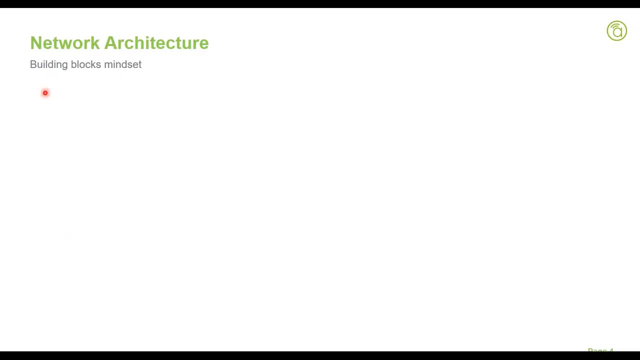 think about it from an architecture perspective And I want to introduce something like: it's really a building block mindset. If you want to have a really solid architecture, no matter how big or small the job, it needs to be scalable and it needs to be modular. 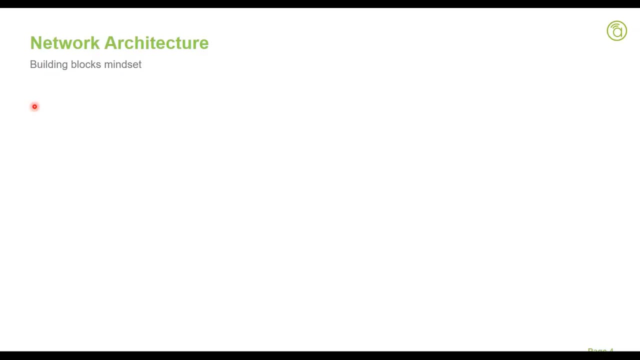 So I'll introduce kind of like a framework to think about for you guys. So we start with the ISP. So this is an ISP building block, So it starts with what you're getting in that house or what you're getting in that small business, Is it? you know, is a Spectrum service. 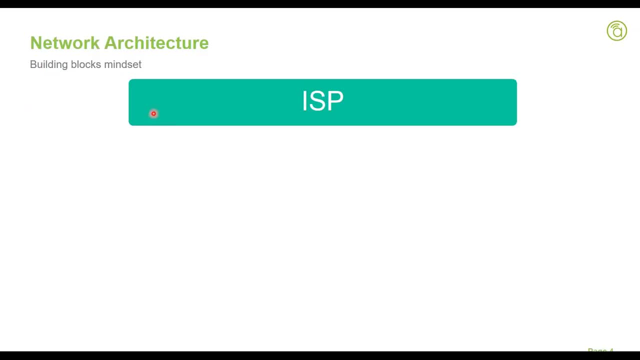 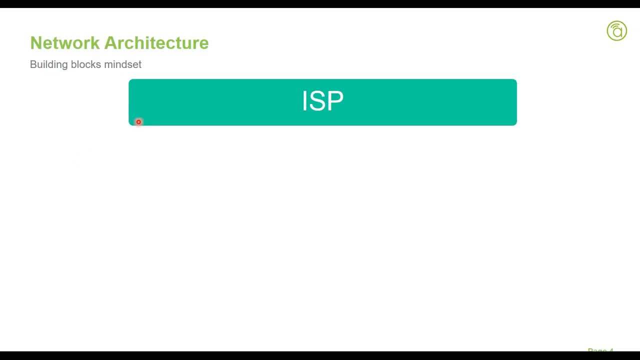 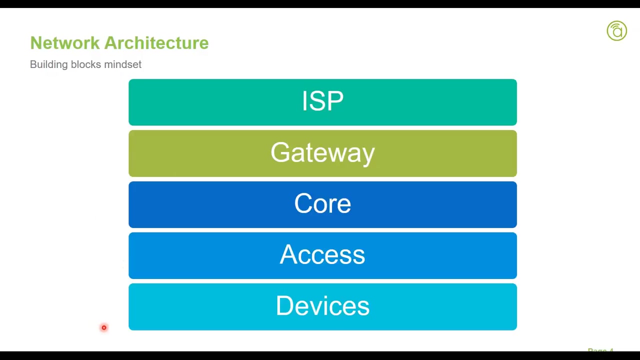 계속 than the devices. So the devices are the edge devices that will interface with the network. So these are your mobile phones, these are your tablets, these are your control systems, your VoIP phones. So this is what the end customer will interface with and will utilize. 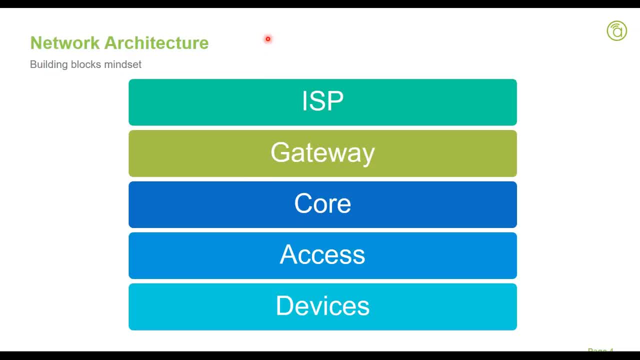 And this is how the traffic flows from top to bottom. So it goes from the ISP to the gateway, to the core, to the access to the end devices. But also, this is how the devices communicate with each other. So they go from devices to access to devices, or devices core to devices. 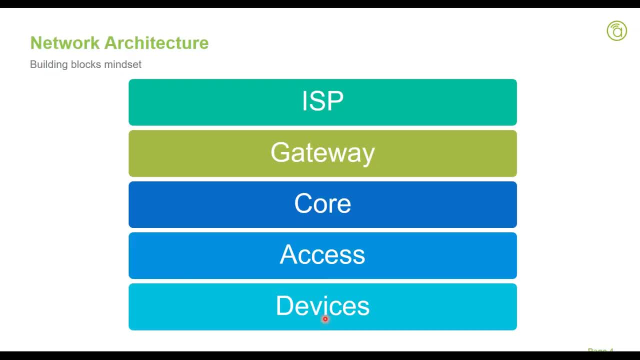 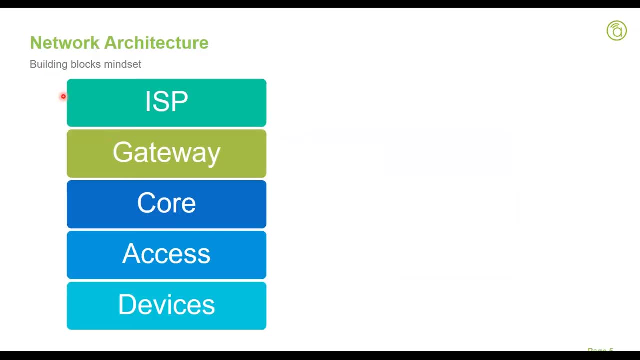 or devices gateway to devices, And that all depends on what kind of setup, how big the network is, if you have VLANs or not. So this is the framework that we would like to establish in your mindset when you start designing, And this is how it translates to a typical 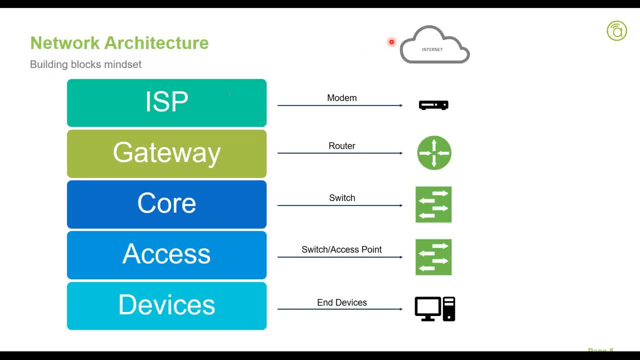 traffic path. So if you think about it, you know traffic coming to the internet or from the internet. it goes through typically a modem, and that's usually a third-party modem from the ISP, then goes to the gateway, which is a router, then goes to a core, which is a core switch. 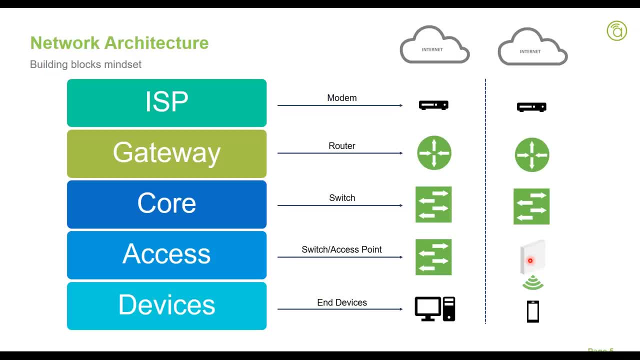 then goes to an access layer, which is either an access switch or, in case of Wi-Fi, we have access points And then that interface with the end devices. So this is the framework and this is how we should dissect the network. So let's take an. 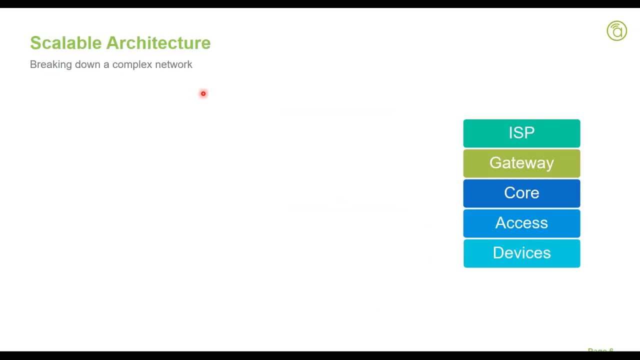 example of you know. I want to say it's a typical network job that you deal with on average. So on average we see from our customers that they will have between 50 to 100 devices on a typical network. So this starts with a lot of end devices. So those devices would be, you know, control touch. 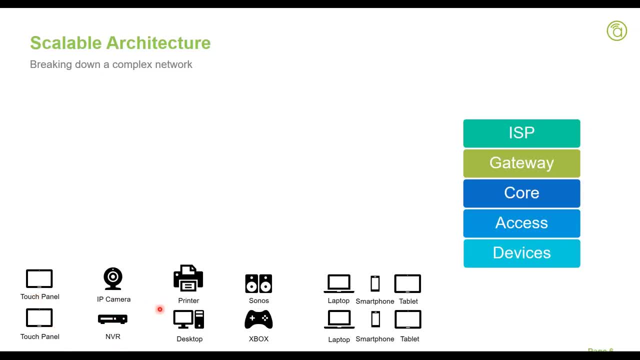 panels, a lot of IP cameras and NVR, a couple of printers, a couple of desktops, some Sonos or some you know, wireless streaming service, a lot of entertainment TVs as well. You get a lot of personal equipment. 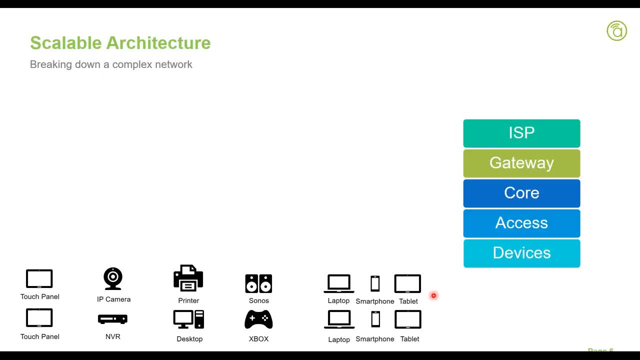 like laptops, smartphones and tablets. We see now- and I'm guilty as charged- it's like every individual in the household will have at least two of these three, if not all three or more. So you will be surprised on how many devices on a typical network will be, And I see on average it's between 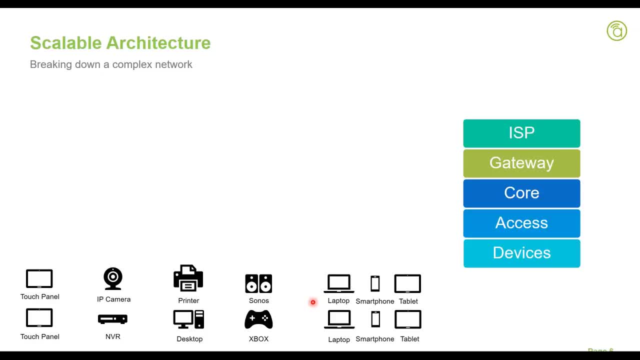 50 and 70. So this is a typical job and this is the devices layer or devices block that is here. So here's how we want to. you know, if somebody you know you sat down with a customer and say: 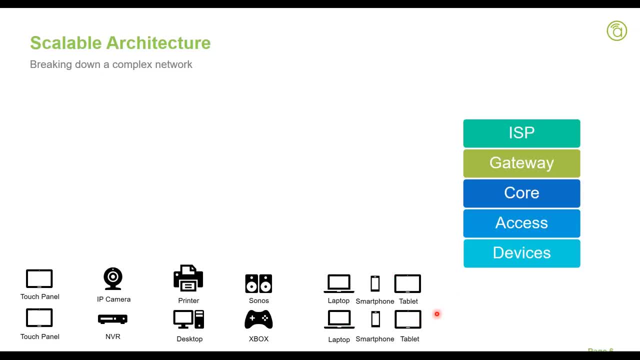 it's like I got- I need all of these things in a new job And you start to dissect this network. So you start with the internet, so you know it's coming through a cable modem and now you got this cable modem that plugs into our 300-inch. 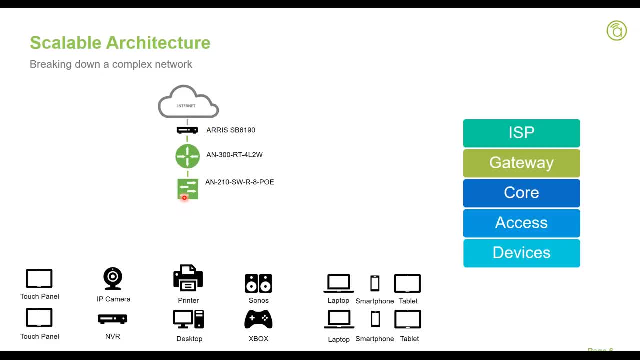 300-series router, Then you got a 210 PoE switch. Then that 210 PoE switch as a core switch connects to a lot of access network devices includes PoE switches or unmatched switches or access points. So from an architecture standpoint this is what we call hub and architecture, or a router on a 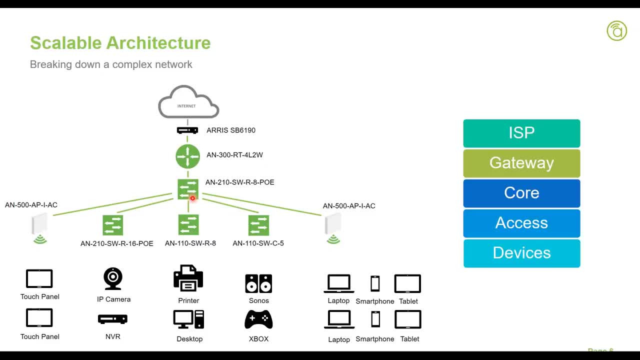 stick architecture. So the switch is the center point, the core switch, And this is a scalable architecture because now this eight-port switch can connect up to eight access devices. So if you have eight switches or eight access points or a combination of both, you can get up to eight. But let's say 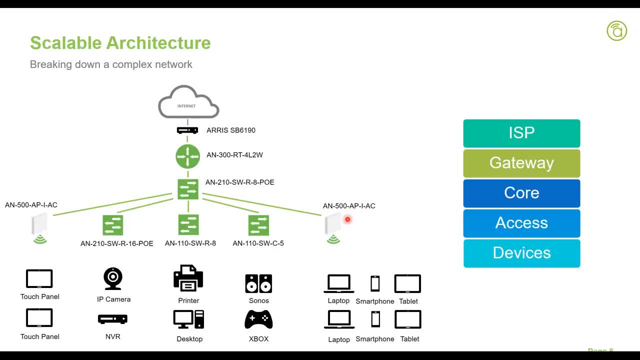 you know, the house or the network expanded. they installed three or four TV locations in the future. and now you are. you know you're bottlenecked by the number of ports on that switch. All you have to do is come back to the job, swap this core switch and you're good to go. 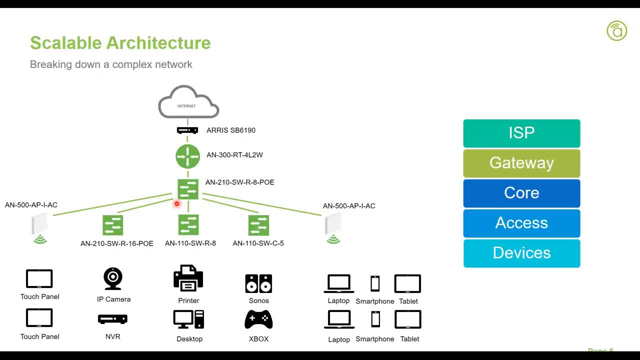 So you can do a core switch with a 16 or a 24-port switch, and now you can expand your access layer to more than to about 24 access switches or access devices. So this is how you can scale this architecture, because you are bounded by the number of ports on that core switch. 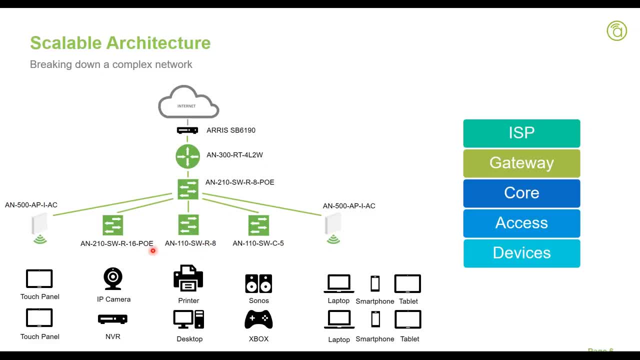 So same goes into those edge switches. So let's say, say we have an eight port here, an eight PoE switch port, then you connect up to eight cameras to it, So you're powering eight PoE cameras on this eight PoE switch. 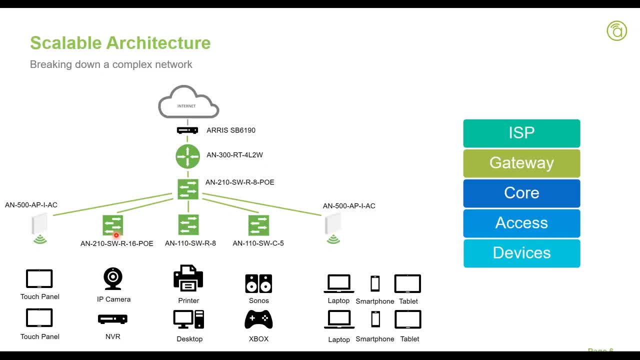 And two years down the line, the customer comes back and say, hey, I want to install a couple of cameras in the front or in the back of the house. And you say, right, I populated all my ports on this access switch. 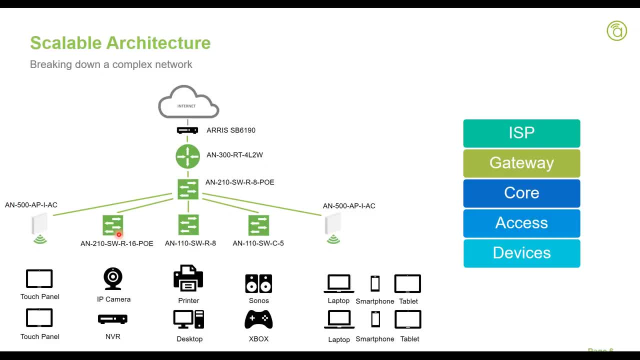 So, Mr Customer, in order for me to expand these cameras, I need to expand the PoE ports on that switch. So all I have to do swap the eight port with the 16 port And this way it's one component change in the network that expands your doubles the. 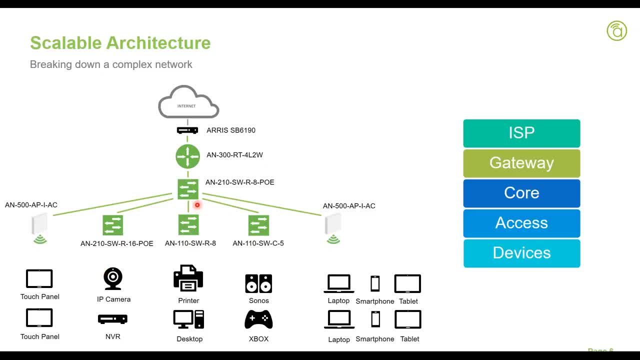 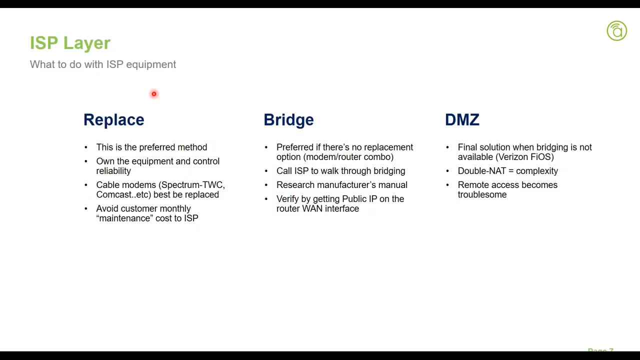 capacity of your IP cameras. So I will go next, layer by layer or block by block, and see and share with you guys some of the tips and tricks for each of these. So we start with the ISP layer And this is what we talked about as the modem. 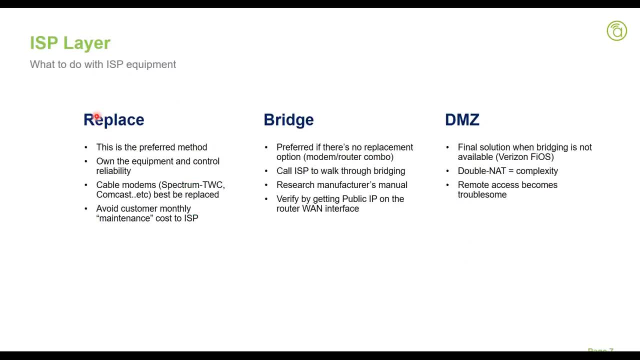 Usually comes in a separate box. Really, when it comes to modems, you have three options: Either you replace, or you bridge, or you DMZ. The replace option is our preferred method And this is something that we recommend to all dealers, if possible, whenever possible. 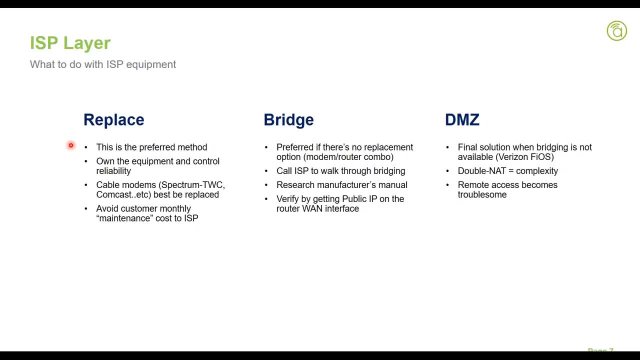 swap out that modem that comes from the ISP with the modem that you own. So this way you can get the higher quality modem and you can guarantee its performance and you own it. What we saw is that for cable modems, for example. so we are here in the North Carolina. 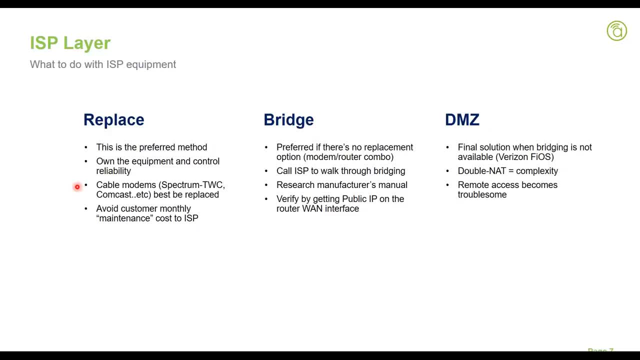 area, or even in the Midwest, when Spectrum, Time Warner or Comcast, it's really preferred to swap those cable modems with the ISP. Okay, And that is something that I did not as a customer, I was on a trip with somebody and I went to the market and it was really great. 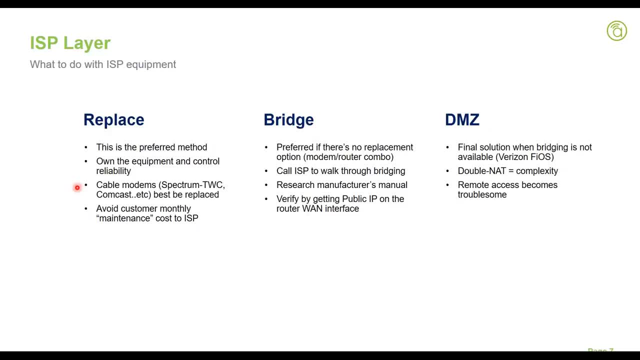 I was just sitting in the middle of the market and I was like, okay, here is my thing, I'm going to buy this thing. I'm going to buy this thing. I'm going to do that. It just comes in this box. 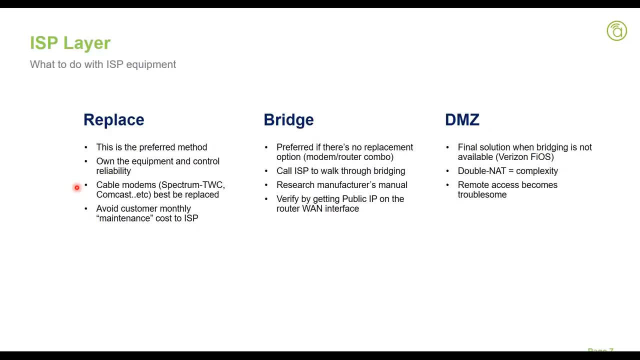 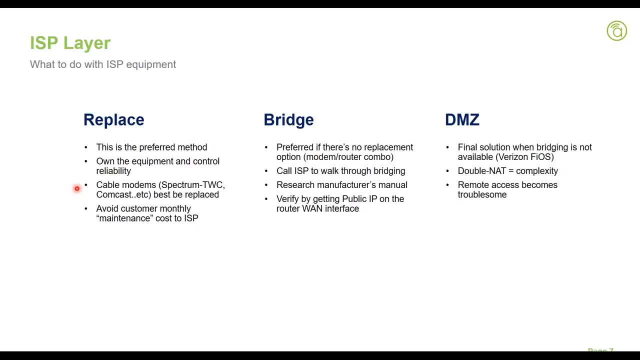 Very reliable. It needs to rebooting every once in a while but overall it's much better than what you get from the ISP. But also the way you can sell on the customer is that almost all those ISPs when they put their modem in the house. now they're moving towards a recurring cost, or they call it. 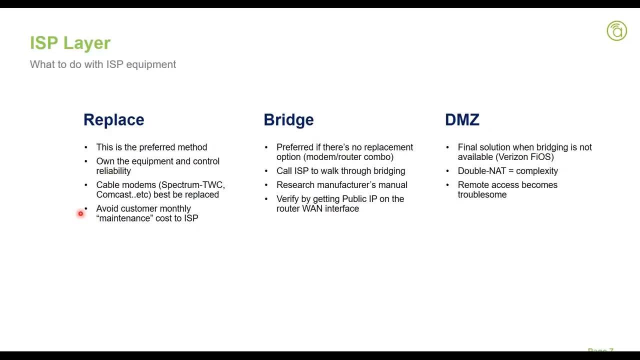 a maintenance fee so they can maintain it and do some firmware updates on it, And they charge the customer about $6 to $8 a month in order to maintain it. So that's a perpetual cost for the end customer. So replacing this modem with one time $110 or $150 modem, it will pay for itself within 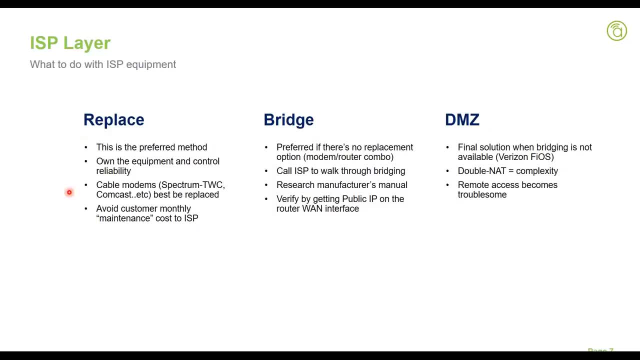 a year and a half to two years tops. So that's something that's very important and we prefer this method. But we recognize that sometimes you cannot replace that modem because it comes in a combo. So the modem is embedded in a router combo and there's Wi-Fi in that. 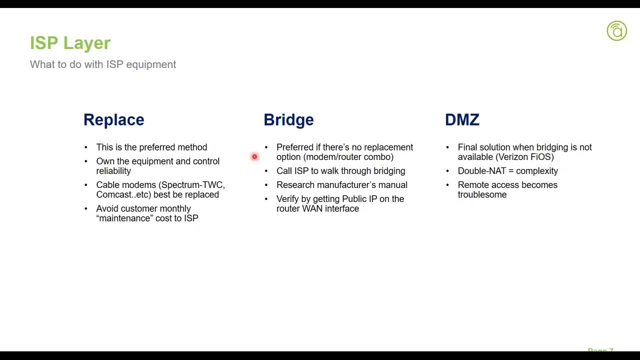 It's a lot worse and a lot more tricky to replace. So what you will do in that case? if there's no way to replace it, your best second option is to bridge it. So keep the modem or the combo from the ISP and bridge it. 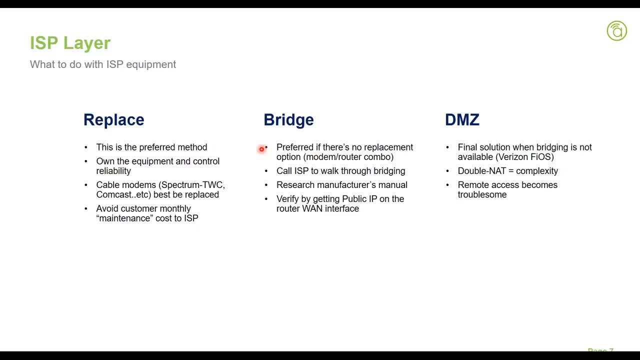 Basically, it will act as a pass-through, So all you have to do is just make sure that you get the make and model of that modem. If you don't have that combo, call the ISP and tell them that they support the staff and tell them that you want to bridge it. 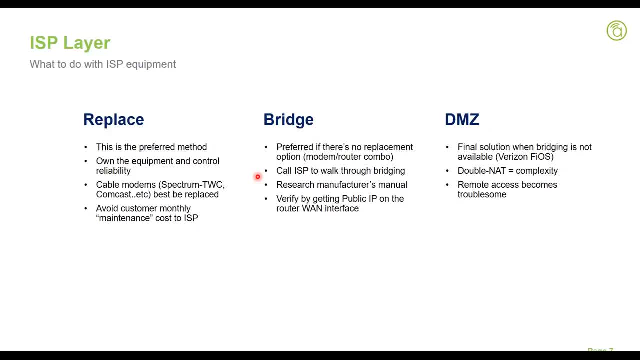 Sometimes it's not fun to work with the ISP tech support, so you might want to resort to do some quick online research in the manufacturer's manual- because most of the time these are well-known companies- and see how can you bridge that modem combo and bypass it. 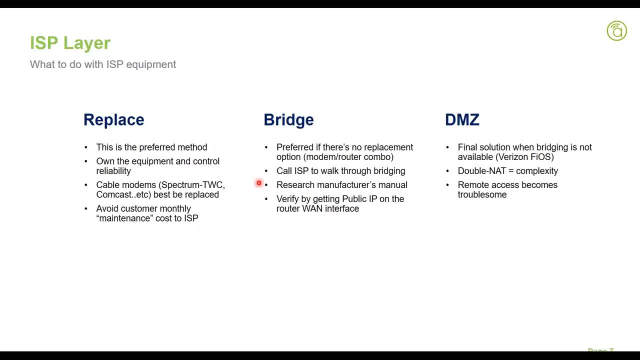 If that combo has also Wi-Fi in it, it's advisable to turn off Wi-Fi in that device, because usually it's not in an ideal place to have a Wi-Fi device in it. How you can verify with this option is when you plug in the router inside that combo bridge. 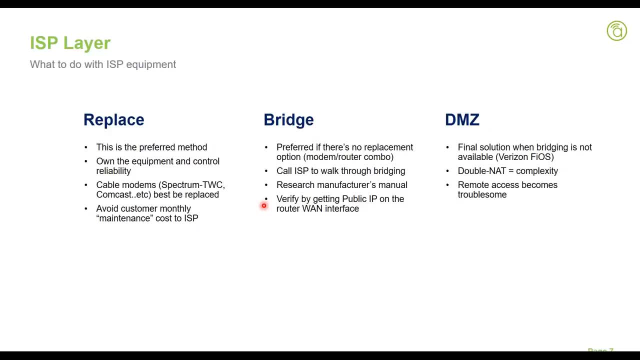 you should see a public WAN IP on the WAN interface of the router. So this is how you verify that this combo modem is working. Now, in the third case, which is you can't replace the modem, you have to deal with it. 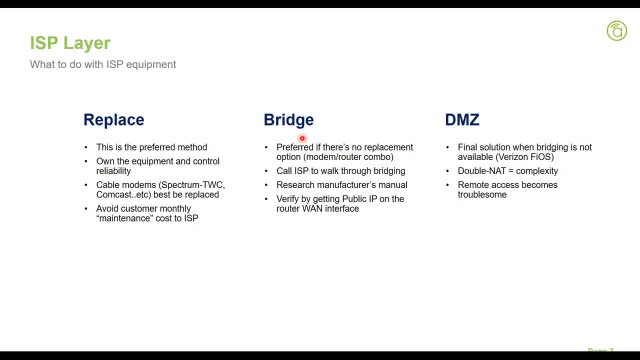 but for some reason you cannot bridge it. You can't find the option. You call the ISP and they said there's no way around it. You did some online research and you couldn't find anything to bridge it. The third and final resort that we recommend to dealers is to put it on DMZ. of that combo. 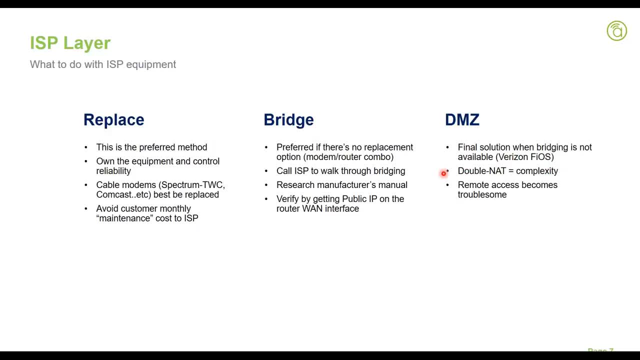 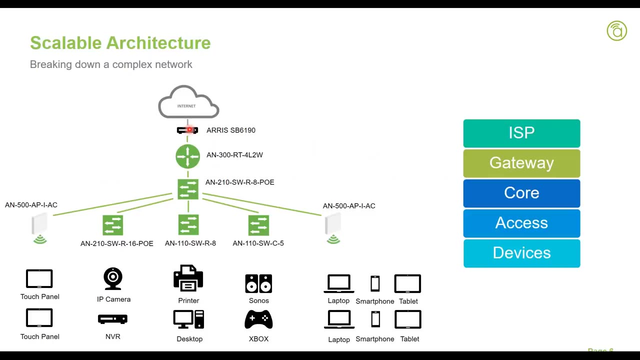 device. We've seen this with Verizon Fios. The problem is that you have to be aware of double NAT situation. Basically, if you go here, the WAN interface of the router is getting a private IP from that combo router. So basically, there's a mini router here in the cable and it's having a private IP to. 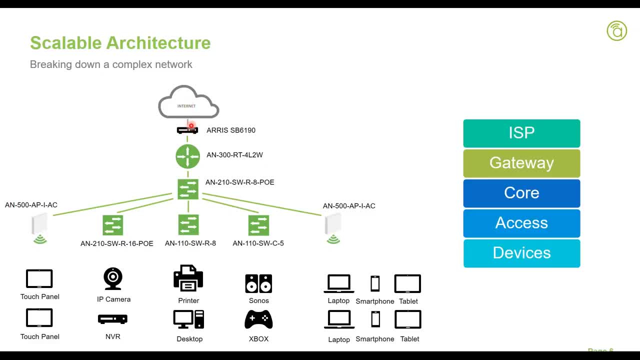 the router and it's getting a public IP from the ISP. So this is a NAT device, so it does network address translation from the WAN public IP to the LAN IP. Then the router will do translation from this LAN IP to another LAN IP. 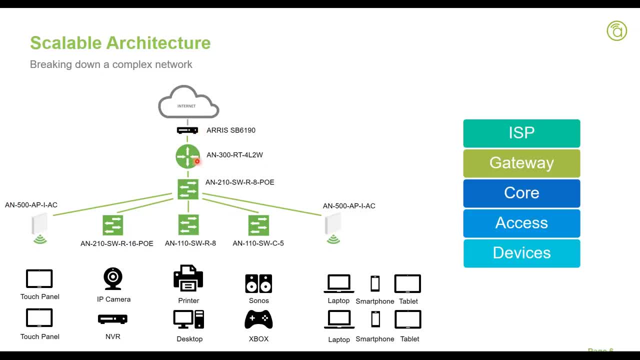 So this is what we call a double NAT situation. The problem with a double NAT situation is that you have to if you want to do port forwarding. it becomes a little bit tedious because you have to do port forwarding on the first NAT device, then port forwarding on the second NAT device. 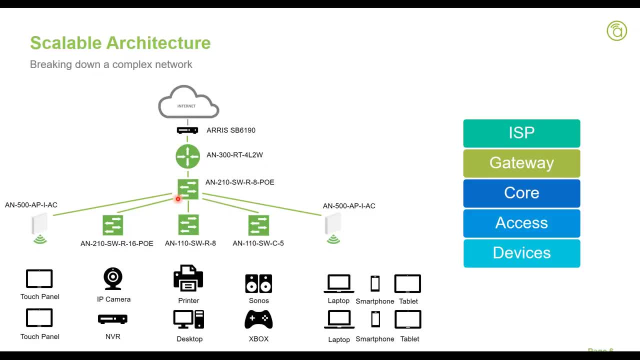 The other problem is if you want to do remote access to any of the devices inside the network, it becomes also problematic because they have to go through two layers of NATing. Now with Oversee Pro and Oversee Hub, that problem doesn't exist because you SSH to Oversee. 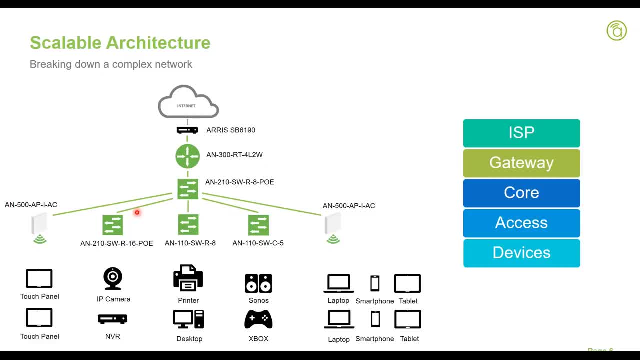 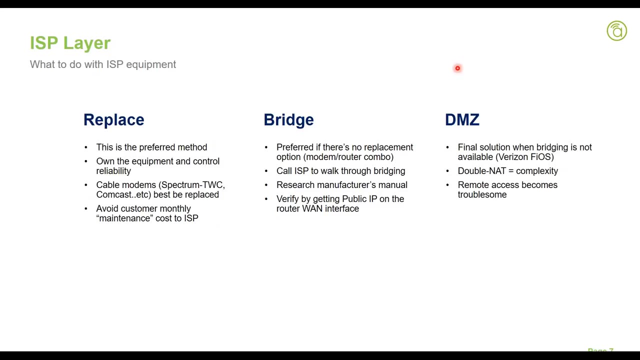 Hub inside the network and you can access other devices, local IP address or local interfaces easily. But if you do not have an Oversee Hub, remote access becomes a little bit tricky and it requires some maneuvering in both the combo from the ISP and the router. 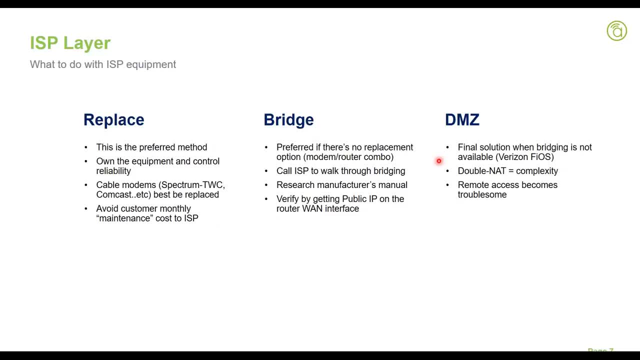 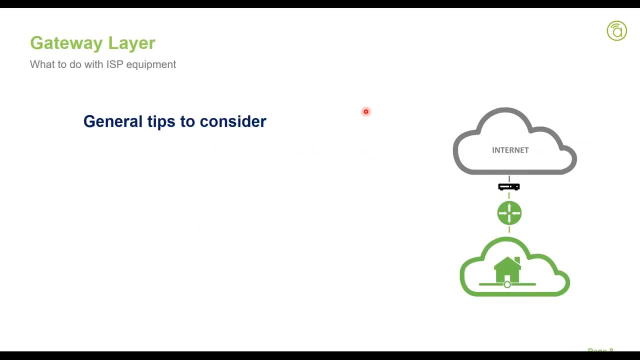 So these are the three options that you have. We have some internal documents in our tech support for DMZing and if you run into that situation, feel free to call our support line and we will help you through it. Now the gateway layer, which is the router. 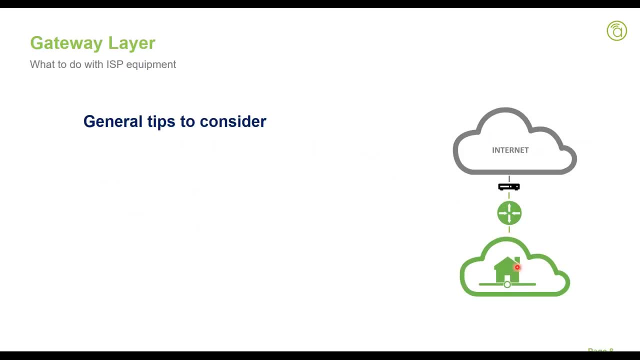 So, basically, the router. what it does is it connects the internal network with the internet. So let's assume that this is the modem that you got and replaced. All it does is it's just a dumb device. Your router is getting a WAN IP address from the ISP and the router is responsible for. 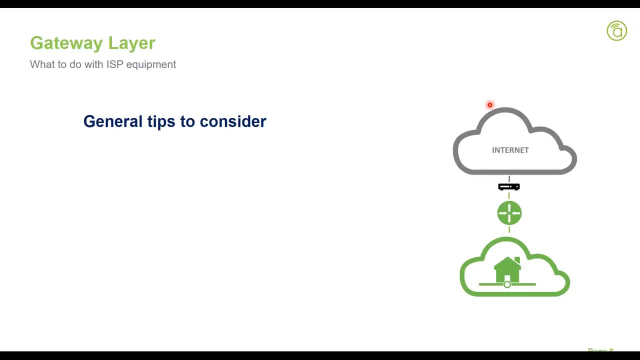 all that translation from inside to outside the network. So here are some general tips and tricks that you can do. Okay, One of the things that you need to be aware of when you think about that layer, the gateway layer, make sure you look at you, spec the right equipment, look at the WAN to LAN throughput. 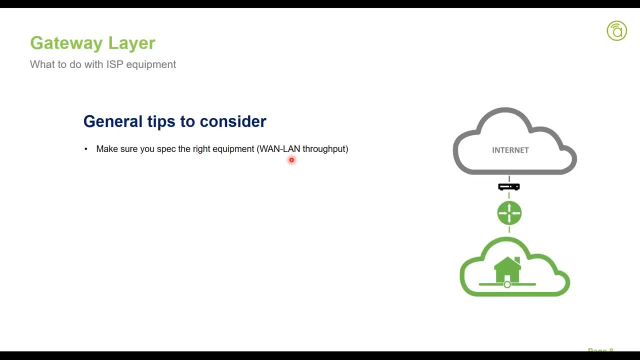 Our current 300 series router is capable of doing up to 500 megabit per second WAN to LAN. I know some of the higher, high frequency questions that I get like: hey, are you going to come up with a higher end router to do one gigabit per second for those Google fibers and the? 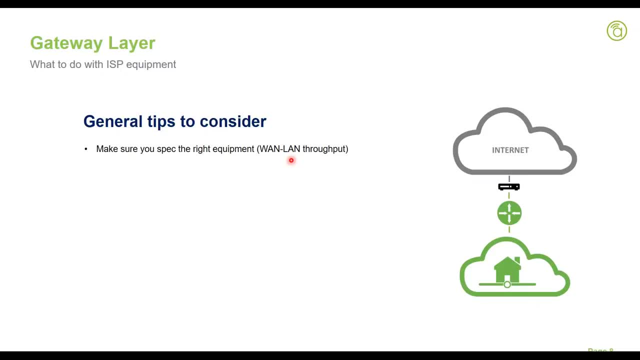 AT&T fibers ISPs. The answer is yes, We are in development, but stay tuned for more information on that. The other thing that we start to see is that some of the dealers are more concerned about your security, and we start to see some of those unified threat management appliances. 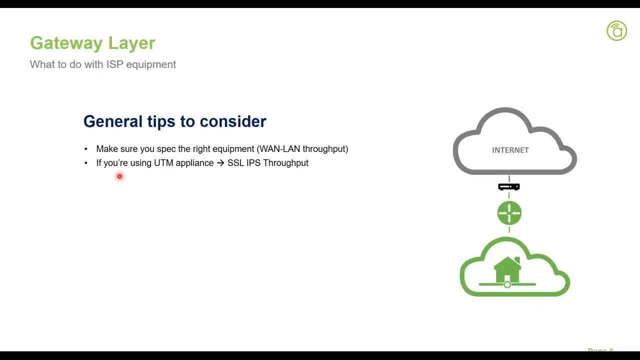 being specced as the gateway device, which is great. This is, Those level of devices are higher. Okay, They're higher than the typical simple gateway in terms of just security. But you have to be very aware that once you enable all those security features, your throughput. 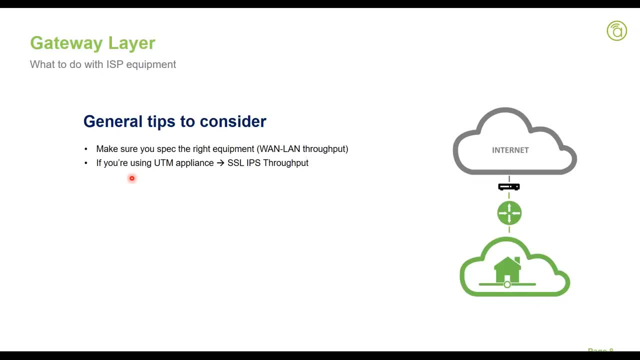 through that device goes way down. So if you go to the spec sheet you have to look at the SSL IPS throughput. So this is basically the UTM device or the UTM appliance is doing deep packet inspection on encrypted traffic, Which most of the modern applications use encrypted traffic to communicate like Facebook. 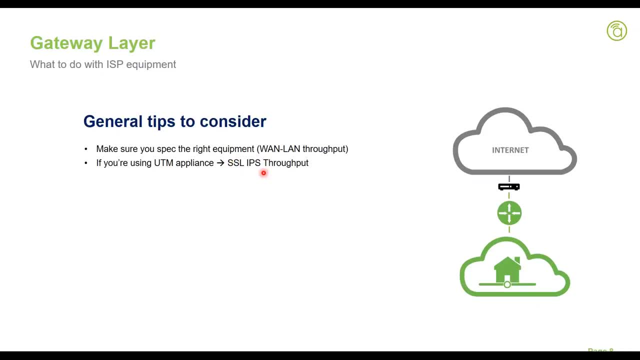 So they have to do a lot of processing on the local device in order to protect the traffic from any malware or any attacks. So what you typically see in a UTM appliance is that, for example, let's say you see a spec that is one gigabit per second firewall throughput. 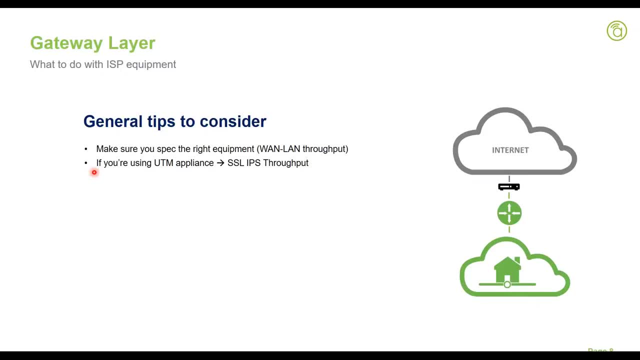 You say great, This is a great appliance. But paying extra attention to the spec sheet, you see the SSL IPS throughput is about 50 megabits per second. So there's a huge drop between not having security features and having security features. 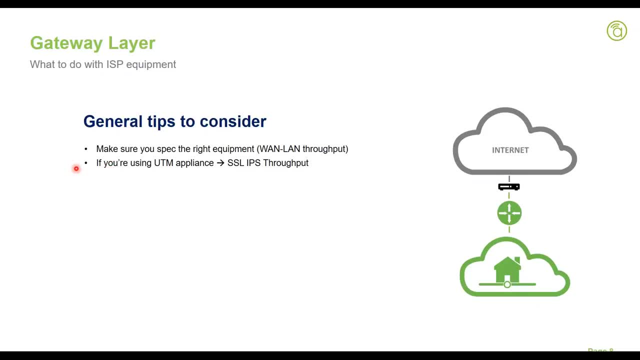 So just be aware it's a good approach. Just be aware that you have to spec higher end equipment based on SSL IPS throughput, Think. last time I checked with one of the dealers. he was looking at a company called SonicWall And he was trying to see if SonicWall will have a good solution for his application. 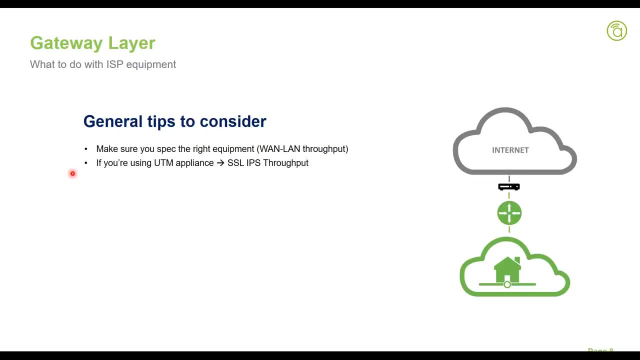 And we looked at the highest end model from a low end series. It dropped from 1.5 gigabit per second firewall to about 200 megabit per second SSL IPS throughput And that equipment cost him on Amazon about $1,800.. 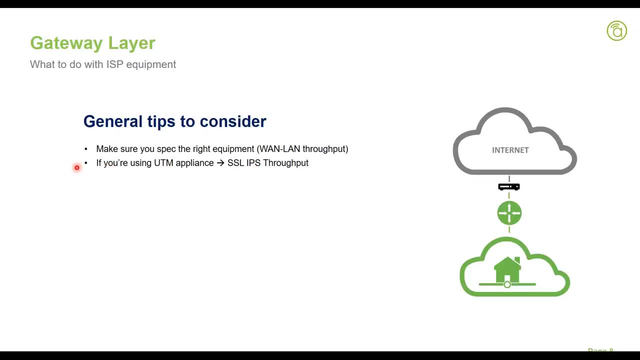 So there is cost associated with a UTM appliance. Obviously it's higher cost than non-UTM appliance, And there's also a performance degradation problem that you need to be aware of. The other thing that you need to be aware of is- or we highly recommend is that use. 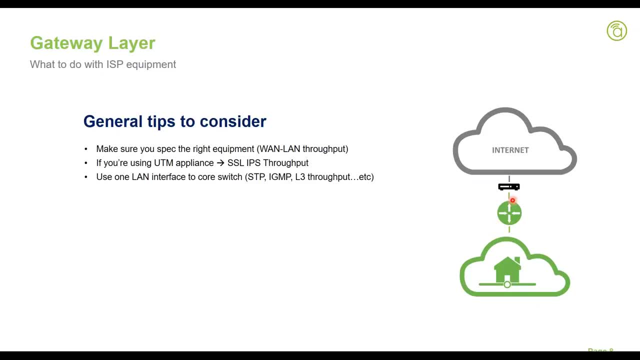 one LAN interface to the core switch. So this is what we call the router on the stick. architecture or design. So basically it's the local network and you have the router sitting on one stick, which is one. It's the interface to the network. 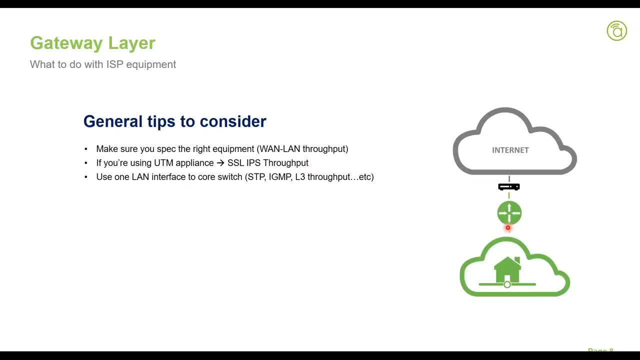 Why we recommend this architecture, even though the router has, most of the time, more than one interface on the LAN side, is because a lot of those routers are not meant to handle LAN traffic properly. So a lot of those routers do not have spanning tree configuration. 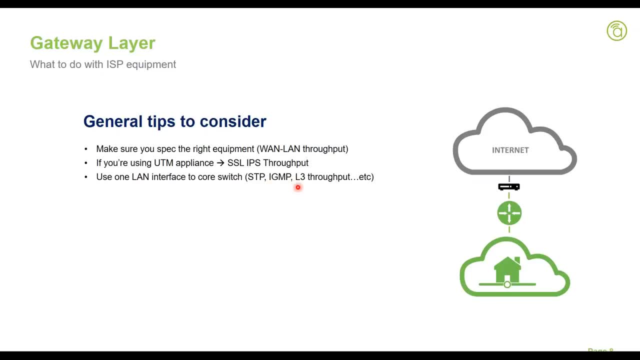 A lot of them. they do not have IGMP configuration. There is, You know, LAN to LAN throughput. there are two ways to measure LAN to LAN throughput. One of them is layer two, which is only ethernet. The other one is layer three, which is IP routing. 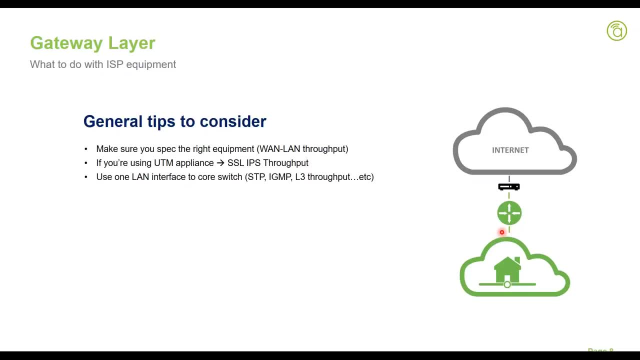 So if you have to do multiple VLANs and you have to do inter-VLAN routing, your IP routing throughput through the router is not gigabit, So you have to be aware of those things when you connect multiple switches to the router directly. So that's why we highly recommend. 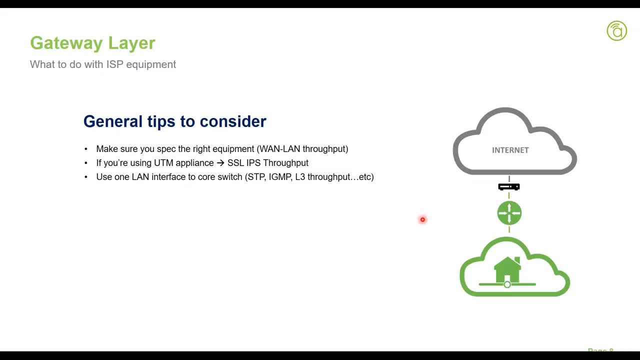 Yeah, We highly recommend doing router-on-a-stick architecture. The other thing that we recommend, since we're talking about routing, you talk about IP subnetting, So standardize on your own IP schema and document it. This is a very, very important thing. 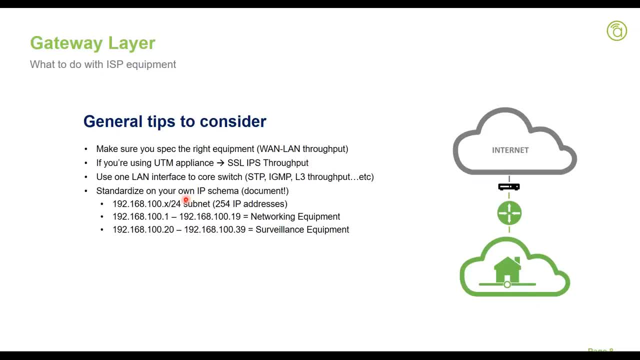 It will make your life 100 times easier in the future. So here's an example that I'm using. It's just an example. First of all, stay away, or I would recommend to change the default 192.168.1 network, because 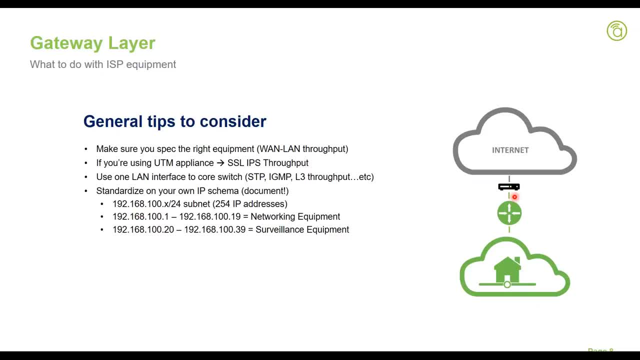 you end up with a lot of default network coming out of the box, maybe on the ISP combo box or when somebody's VPNing into the network. So it's highly advisable to change your default subnets. So let's say, I change my subnet to 192.168.100.x. 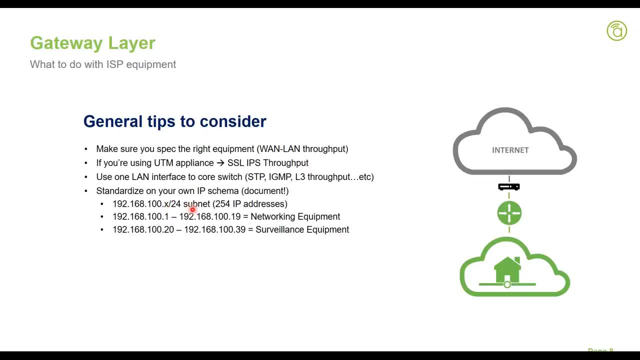 It's a slash 24 subnet That will give me- Yeah, Yeah, It's gonna give me- up to 254 IP addresses. There's plenty of devices that I can connect to this network. So an example of standardizing on my own IP schema is: I say, hey, every job that I go. 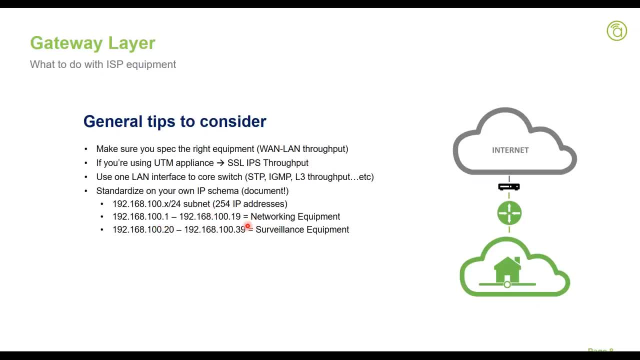 to the range from .1 to .19 is reserved for networking equipment. So this is: .1 is the router, .2 is the core switch, .3 is another switch, so on and so forth. So these are the management IP addresses for those networking equipment. 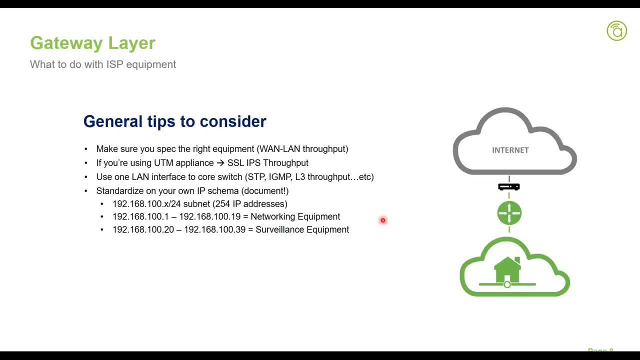 And I standardize. I standardize on those across all my jobs. So if I have to remote access or I have to local access, I don't have to waste time going through documentation or going through some previous notes on what the IP address of that. 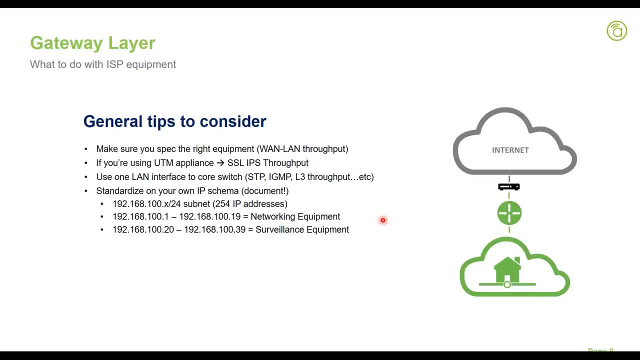 device is. I know exactly what it is. It's always .1 for the router, it's always .2 for the core switch, it's always .3 for the edge switch, and so on and so forth. Here's another example from the IP schemas. 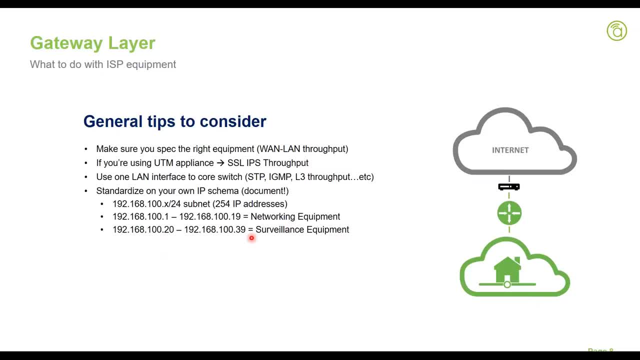 I will start my schema. I'm gonna. I'll start my surveillance equipment from .20 to .39.. That gives me about 40 IP surveillance equipment And I can say I always start with the MVR. so .20 is always the MVR, .21 is the first. 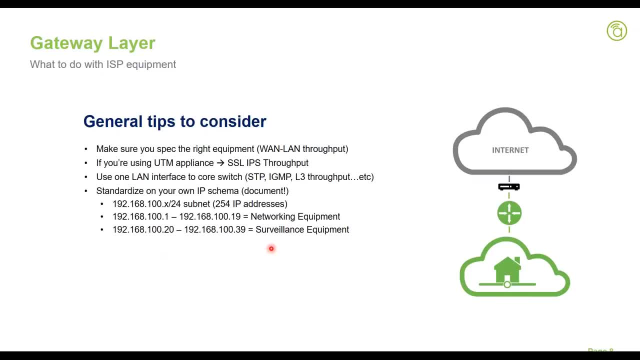 IP camera .22,, .23, so on and so forth. So that makes it standardized and that makes it also very, very easy to follow in troubleshooting. And once I've done a standardized on my own IP schema, I can also standardize on my port. 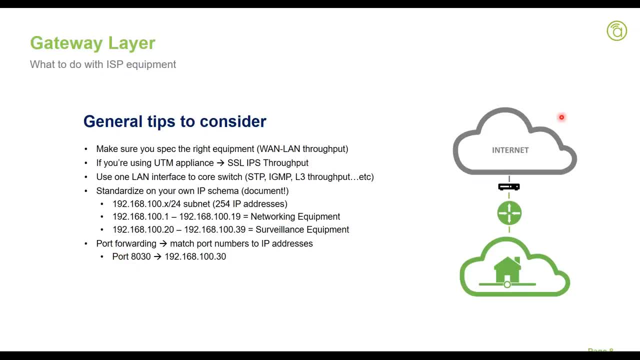 forwarding rule. So one of the very important items is that we highly recommend matching port forwarding rules with IP addresses. So let's take an example of this surveillance IP schema here. So say, between .20 and .39 are my IP cameras and I want to access one of those cameras. 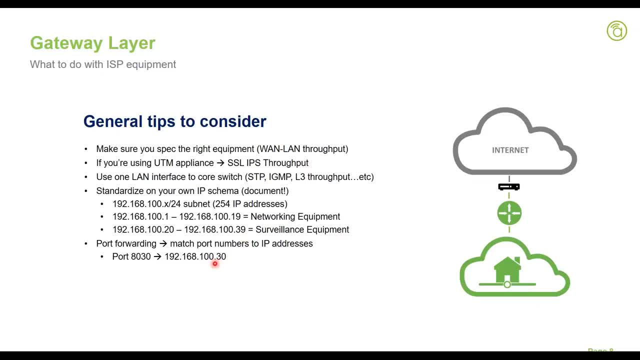 remotely through a port forwarding rule. Let's say I wanna access camera .30.. So one of the best practices. One of the best practices is that I start with a range of ports. let's say 8000 is where I start. Maybe I wanna start at 9000 on the WAN and match the last two digits with the IP address. 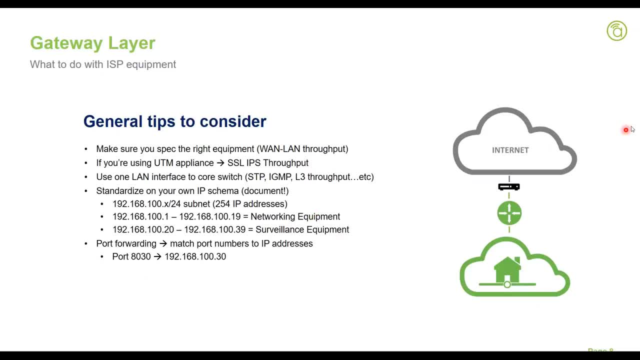 of the device. So let me do a pin here real quick so you can see it. This is 30 matches 30, and so on and so forth. Actually it's the last three digits should match the last three digits here. So if I have a device here that's 130, then my port forwarding rule is 8130.. 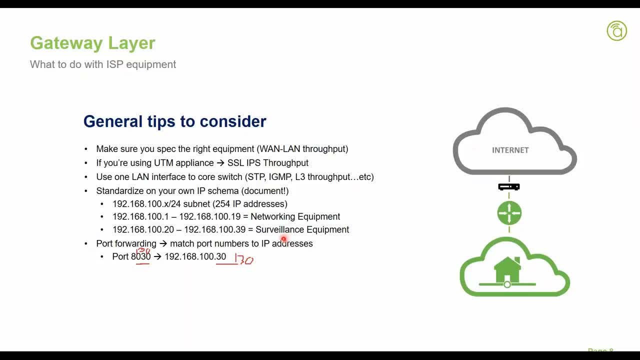 I'm using keyboard, So that's an example of a really best practice. So this way, when you want to remote access to a device, you don't have to even think about it. I know exactly. I'm starting always at port 8000 or port 9000, and I know my IP camera range start. 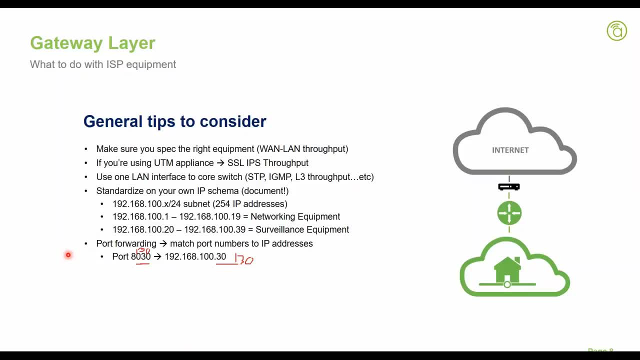 from 20,, 21,, all the way to 39.. I know that I start, for example, north to south. I want to access the third camera from north, then it's gonna be 23.. Port 80, 23 is the WAN or the port that I need to access. 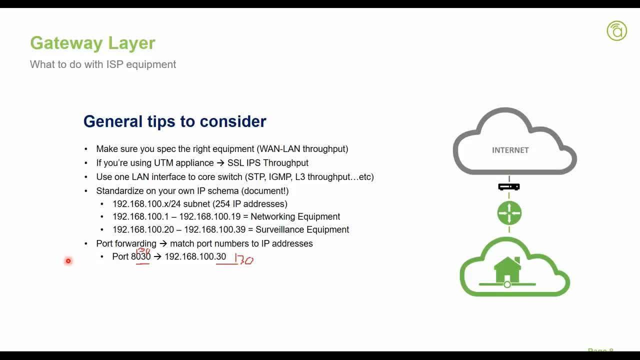 Saved me a lot of time in troubleshooting, just plowing through documentation. The other final tip here is that before final tip is that VLANs you have to consider about inter-VLAN routing. Some consideration when you have inter-VLAN routing and again, if you want to dive into 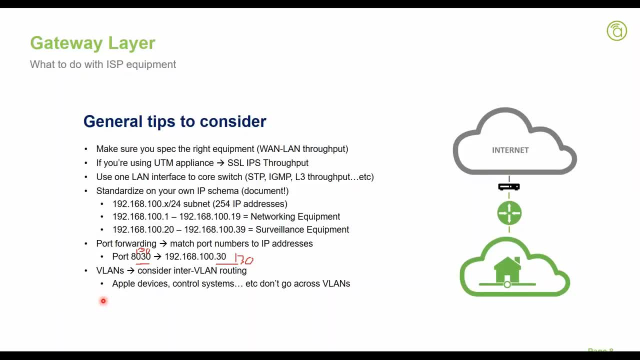 the VLANs. please watch our webinar about VLANs and read the documentation, the support tab. But one important thing that you need to be aware of is that Apple devices- sometimes control systems or streaming services, do not play well across VLANs. 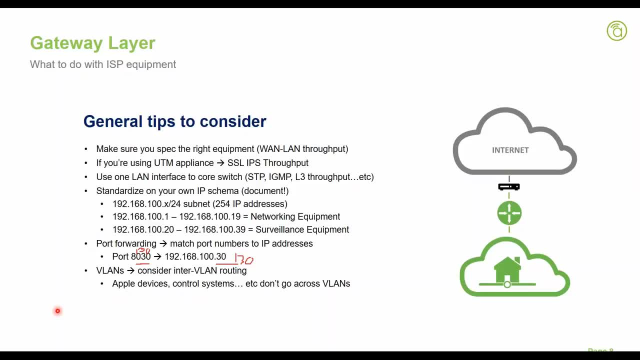 Okay, An example of that: if you have an Apple TV on one VLAN and you have Apple devices like iPhones on another VLAN, your Apple services will not go across VLAN. You cannot do AirPlay across VLANs. You cannot do AirPrint across VLANs. it's gonna be very, very hard. 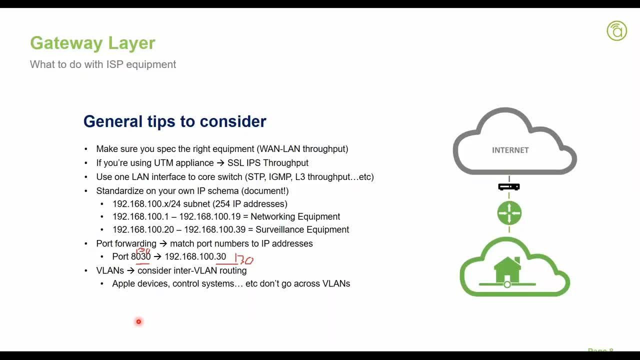 And we found that some control systems also. they don't scan across VLANs because they scan using MDNS. That's technology and it doesn't play well across VLANs. So be very aware when you do VLANs about inter-VLAN routing and inter-VLAN traffic. 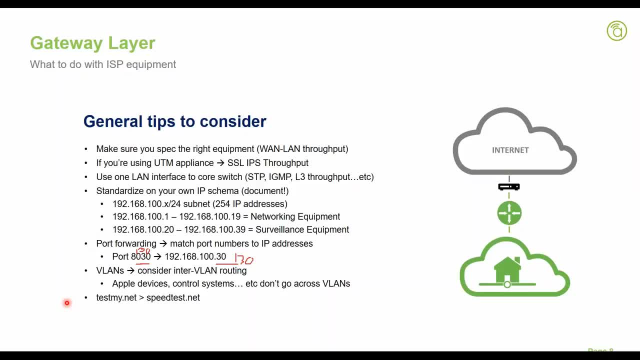 The final tip when we talk about routers is, when you do speed tests, be aware that speedtestnet is not the only tool available for you. It is actually one of the least favorable tools that we recommend for dealers, for a couple of reasons. First of all, it is flash-based, so if your computer is not up to speed in terms of spec, 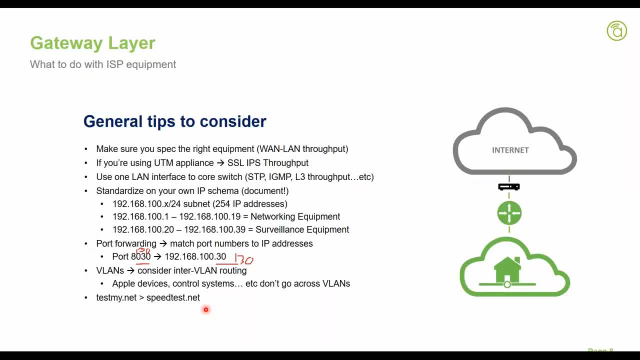 then your computer slows down the speed test. Your NIC card will slow down the speed test. The second reason for speedtestnet is the results vary by the test server. So make sure that you pick or test against different servers in the region and you see. 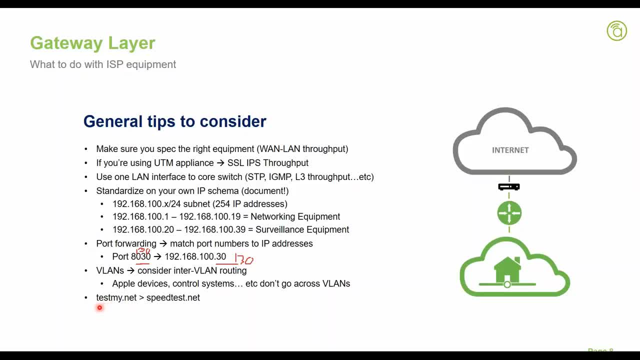 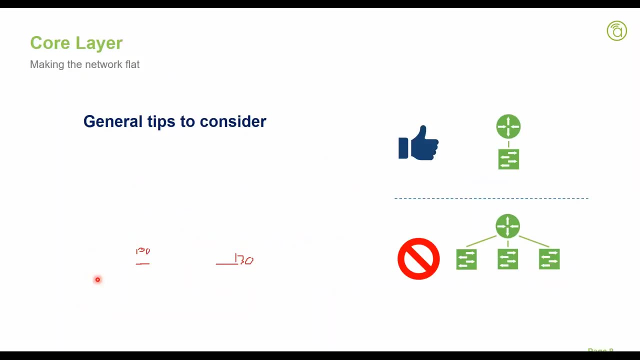 different results there. Okay, So a cool website called testmynet is not flash-based. It gives you an average, an aggregate, about your service. I think this is something that's a good alternative to speedtestnet. All right, Let me clear these drawings. 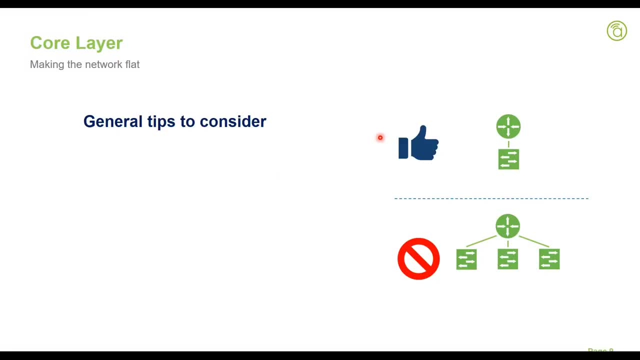 So we go to the core layer And, as we say, the core layer, our goal here is to make the network as quote-unquote flat as possible, Which means that you want to minimize the speed, You want to minimize the number of hops between different segments of the network. 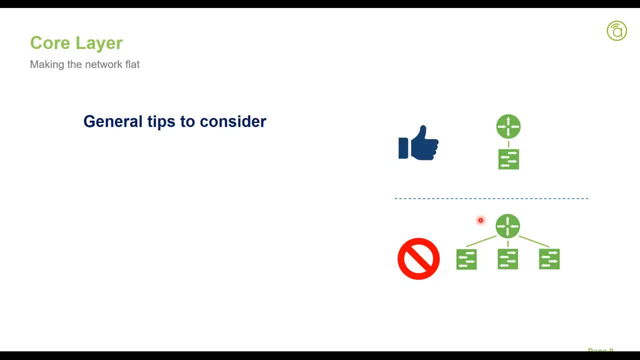 So, like I said, for performance purposes, for a lot of different reasons that we mentioned in the gateway layer, we would like to keep one core switch off of the router and then everything off of that core switch. It is not recommended to use multiple core switches off of the router. 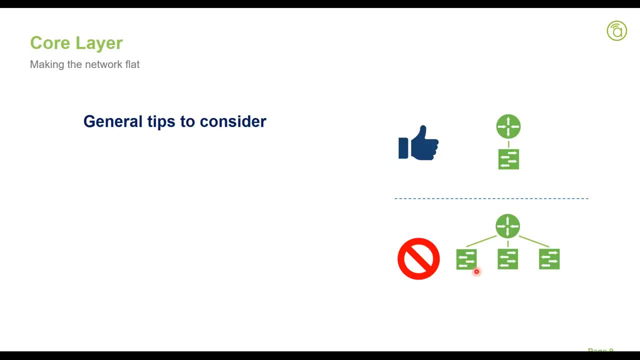 Okay, You might end up using this architecture for really large jobs for various reasons, But if you are designing from the scratch, it's highly recommended to use one core switch off of the router. If you use multiple switches off of the router, you run into issues with IGMP snooping on. 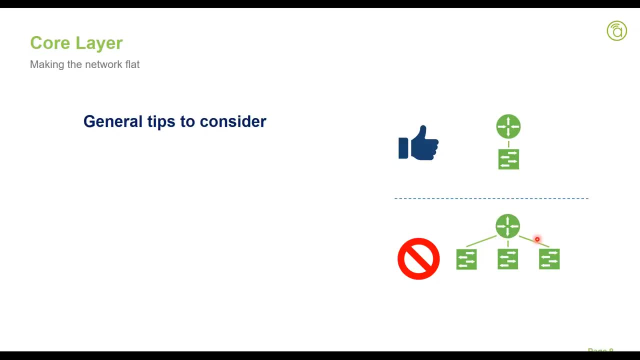 the router. if it's not supported, Spanning tree issues. if it's not supported on the router, your layer three traffic- land-to-land- is going to be less than gigabit per second, So it's really not a good situation. So, like I said, make your network as flat as possible. 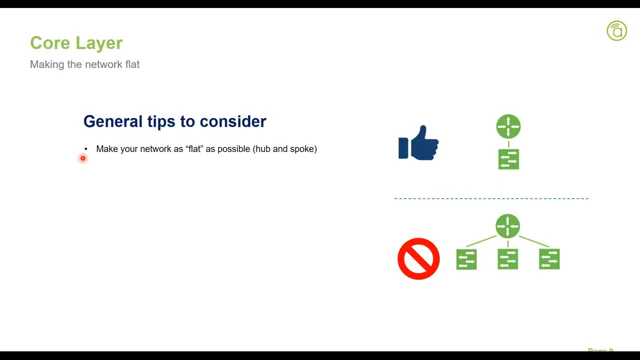 Make it as a hub-and-spoke topology like we talked to, So everything is fed off. that core switch, And in this layer actually a managed switch, is better than an unmatched switch for various reasons And if you watch the spanning tree and Sonos webinar, we explained that. you know the. 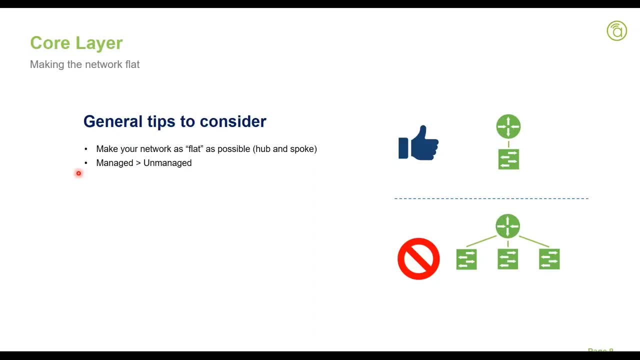 spanning tree algorithm is a little bit more complicated than the core switch, but it is a little bit more complicated than the spanning tree algorithm. So you can control the spanning tree algorithm and you want your core switch to be the root bridge for spanning tree. 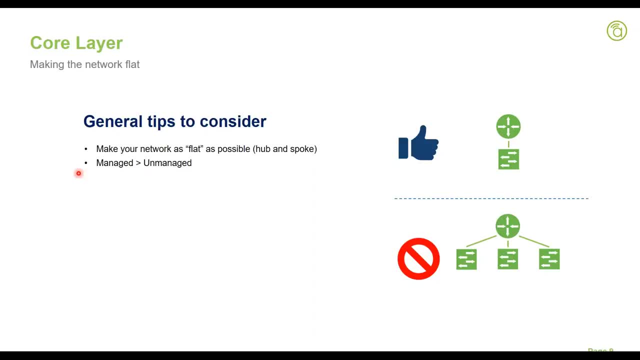 So you want to force the network to get all the traffic through the core switch, not through. Sonos makes sense and it's better than an unmatched switch, And if you have access points in this scenario, I think a lot of the jobs will have access. 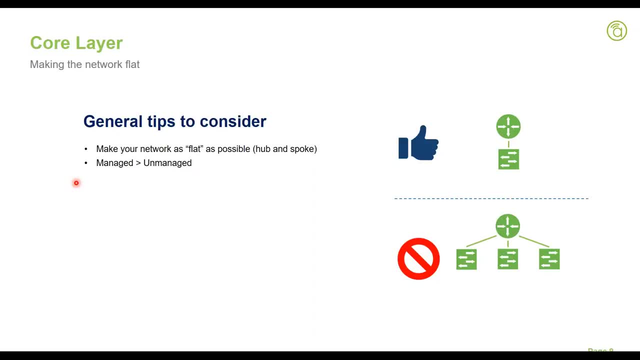 Jobs will have access points. It is also recommended to use a managed PoE switch, And this is one of the reasons that we do not have an unmanaged PoE device is because we would like to keep that control in a managed platform. The other thing you need to think about from a design perspective is: you want to keep your 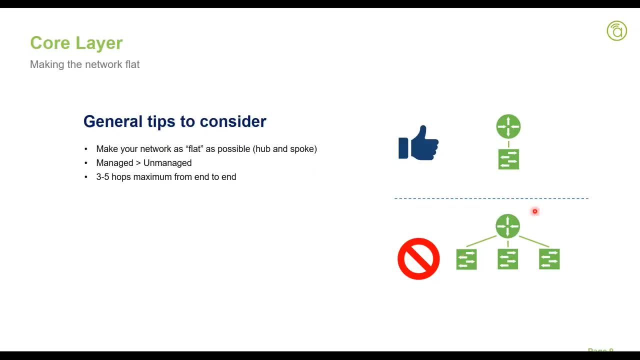 hops. This is the jump. So if your traffic goes from this switch to the router, this is one hop. You want to keep it to three to five hops maximum from end to end- Usually- Usually dealers don't think about it- from device to device. 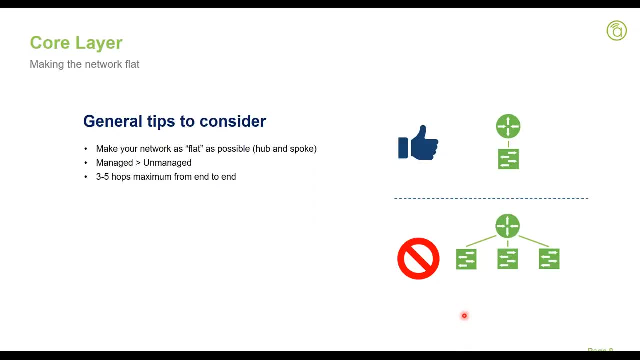 They think about it from device to the internet. It's like, hey, I got three or four hops between my device to the internet. This is good for the internet traffic, but what about traffic going from a control touch panel to the control processor? 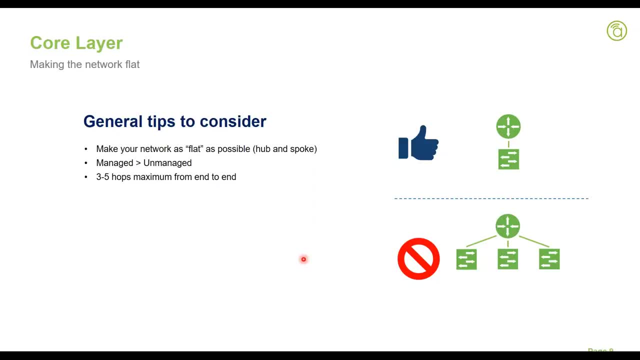 That needs to be between three to five hops maximum in a good design. So that's why you have a flat network. We also recommend from a physical installation to color code different types of traffic if possible and standardize on that. Like I said, if you have access points, use a PoE switch in the core as a core switch and 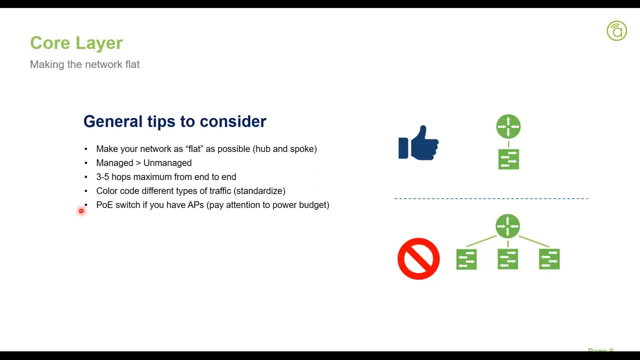 make sure you pay attention to the PoE power budget. So an example for our switches: a 210 has half PoE power budget as a 310. So it depends on the number of access points in the job and depends on the number of PoE. 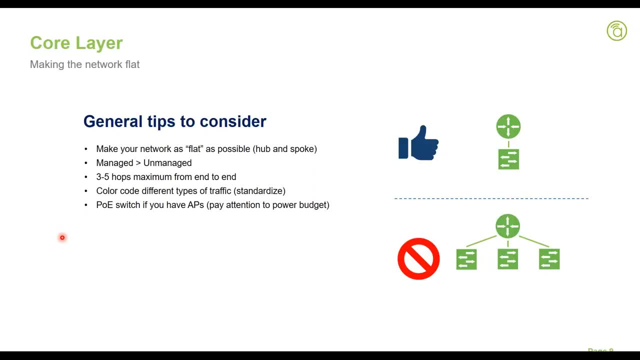 devices in the job, You might want to select a 210 versus a 310.. Like I said, from a spanning tree perspective, especially when you deal with Sonos and we've seen lately some TVs, actually they have some spanning tree problems: the Samsung TV and. 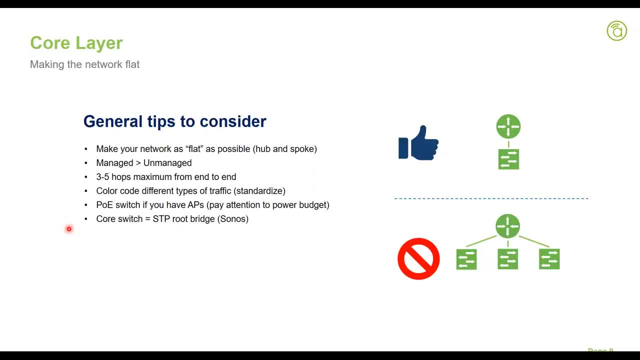 the Sony TV we ran into a core switch needs to be the spanning tree root bridge And when you have really large jobs you need to start to think about V-lanning those shoddy traffic. So if you have a surveillance system, I would start with surveillance and separate V-lanning. 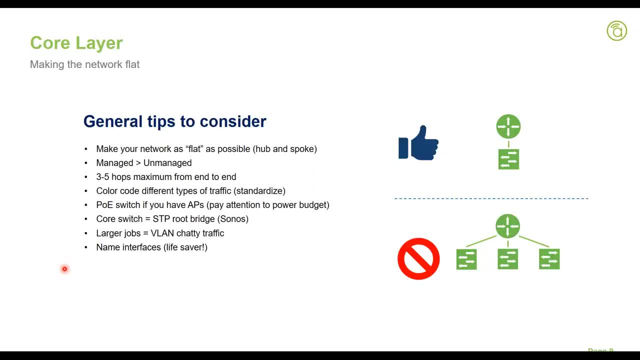 Yeah, And then if you have a security system, I would start with surveillance and separate V-lanning. to begin with, Make sure you name interfaces on that core device, on the core switch. It will save your life when you go six months, eight months after the fact and you want. 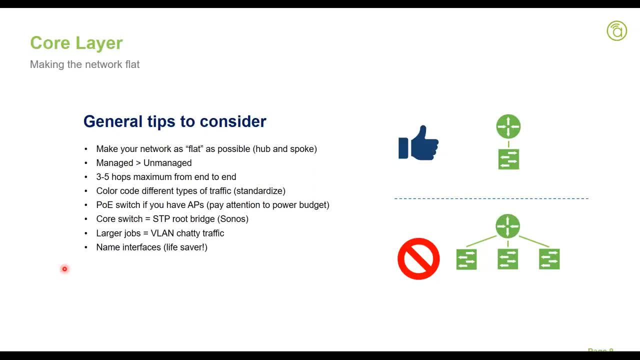 to troubleshoot something. This is when Oversea, as a cloud management free cloud management tool, is very valuable for you. It will take a couple of minutes of your time to go through Oversea and name each interface. Say interface. one is connected to access point upstairs. 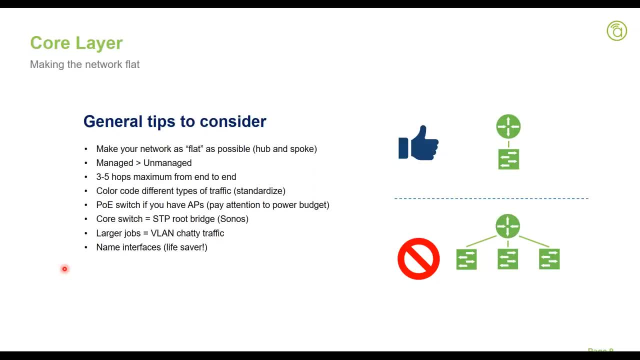 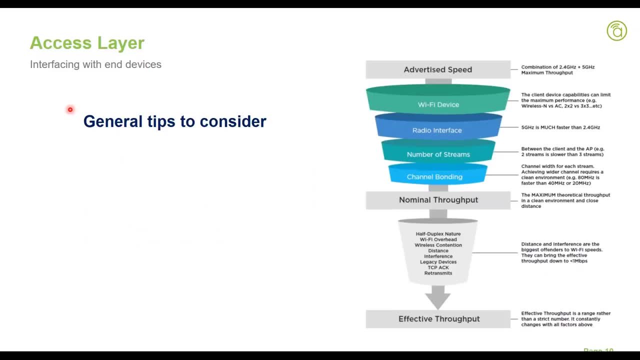 Yeah, Or interface number seven is connected to access point basement. That will help your life a lot. Now we go to the access layer. So the access layer is the layer or the building blocks on the solution that interfaces with your end devices. So that's an interface with your control touch panels, with your Sonos devices, with your 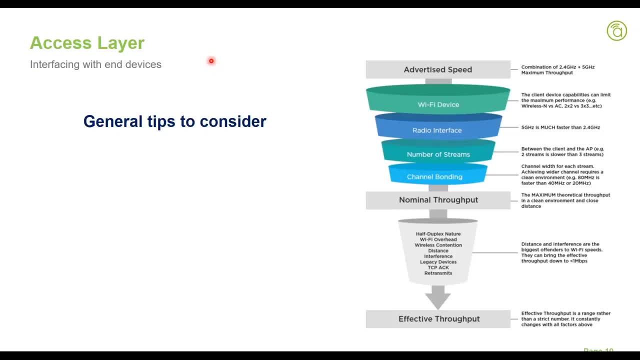 TVs with your end clients, So when they have their laptops or mobile devices. So there is a wired component and there's a wireless component And, like I said in the previous webinar, the last webinar we've done- on the truth about Wi-Fi speed, and this is something we also documented in a blog. 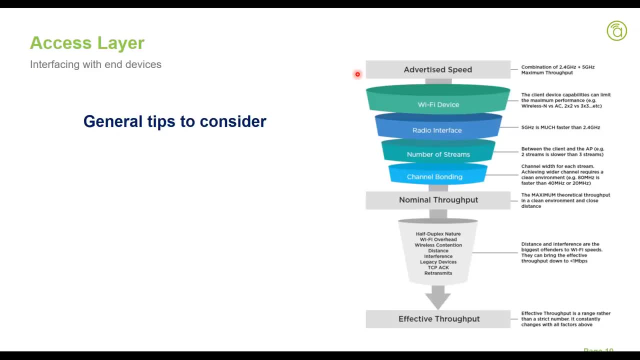 If you go to our blog, there is a big difference between the advertised speed on any networking manufacturer access point and what you should expect in real life. So an example: a 700 series access point that we have, of any equivalent access point that we have, we'll advertise 1750 megabits per second. 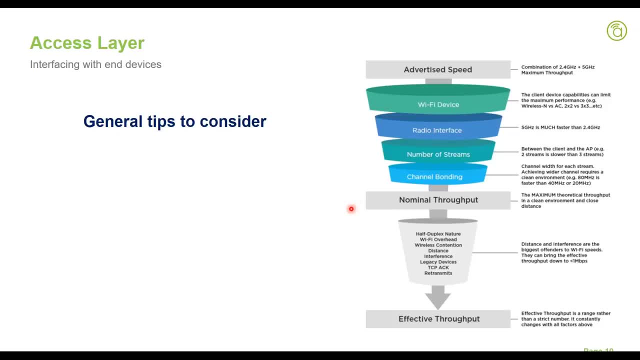 The nominal throughput will be around 800 megabits per second. The effective throughput in real life, based on a lot of variables that you cannot control ahead of time, will be between two to four or 500 megabits per second. So there's a big gap between the two. 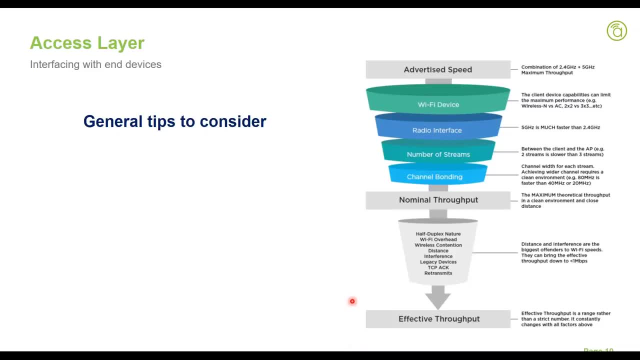 Yeah, Unfortunately that's the nature of Wi-Fi, That's the nature of the standard. There's no special sauce between any different vendors for that. So make sure that you understand those limitations and make sure that you set the expectations right with your customers. 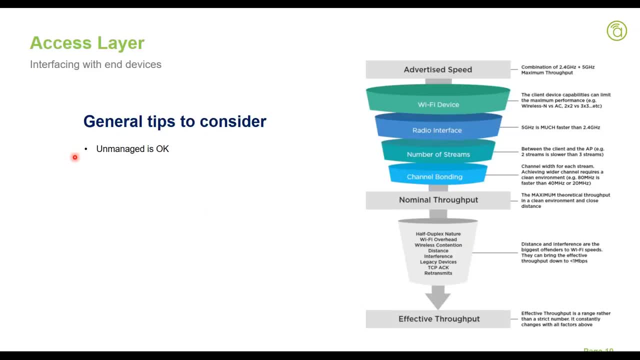 So from the access layer perspective, unmatched switches here they make sense from a cost effectiveness and just ease of deployment And I would account for 20 to 30%. Yeah, So if you have a port expansion in the future for any access switch- unless it's a really 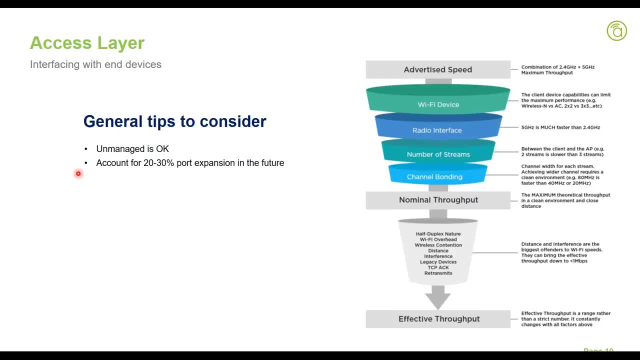 special case. So if you have a PoE switch, for example as an access switch, and you have a requirement of eight cameras or seven cameras, I would not get an eight port PoE switch, I would get a 16 port PoE switch, just to make sure that in the future expansion you are 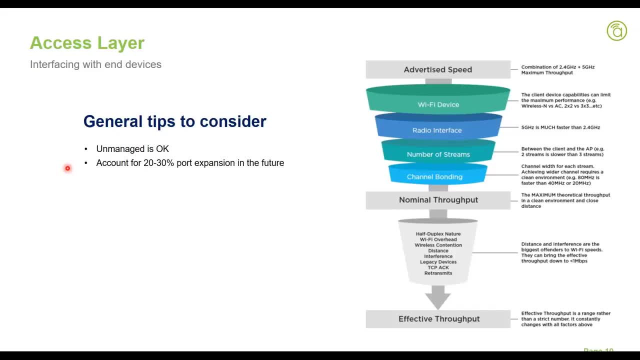 covered. It's really hard for the customer to come back a year from now. Yeah, Yeah, Yeah. So it's really hard for the customer to come back a year from the job. ask for one or two IP cameras to be added and you come up with a quote that you need to swap your switch. 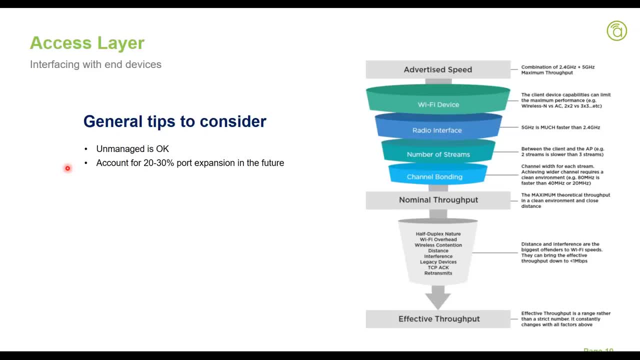 and it's a couple hundred dollars extra, So plan for it as expansion. Sometimes we understand that you need to be on a budget, on a tight budget, so just make sure that you account for that. When it comes to wireless, it's something we stress with our customers, that dual band 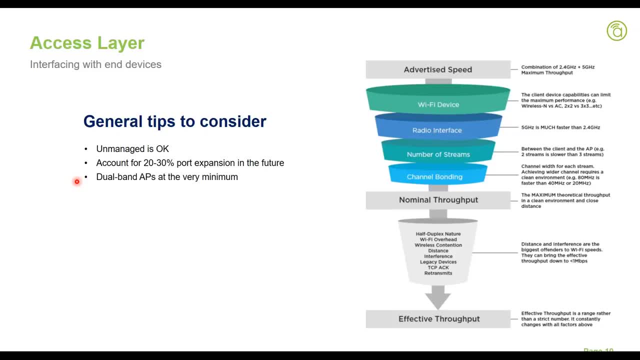 APs 4 and 5 gigahertz APs- much more important than any cost-effectiveness, so I would start with a 300 series access point at the very minimum. it's a dual band 2.4 and 5. the 2.4 gigahertz spectrum is a lost cause. it's really. 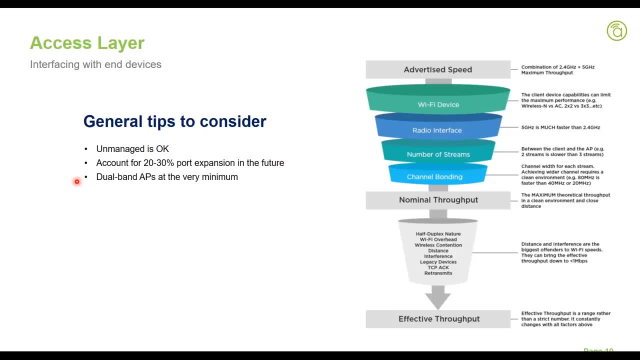 really hard to get any meaningful throughput out of it and it's getting even more scrutiny from the FCC. if you want to plan for the future, wireless AC is definitely the mainstream now wireless and is an old technology. if you want to do analogy for video traffic, wireless AC is the 4k wireless and is 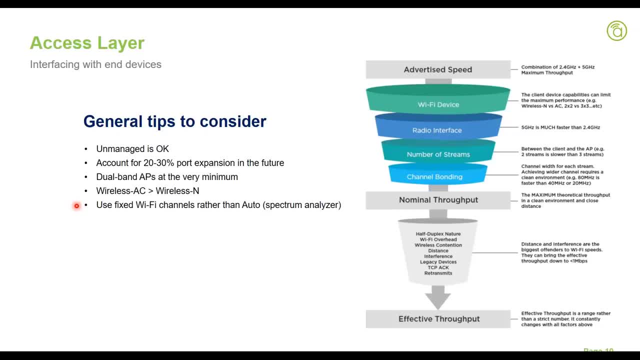 1080p use fixed Wi-Fi channels, so all the access points are auto in terms of channel selection. this is when you your investment in a spectrum analyzer is very important, because if you do your job and you do spectrum analysis and you do site survey on that job, you 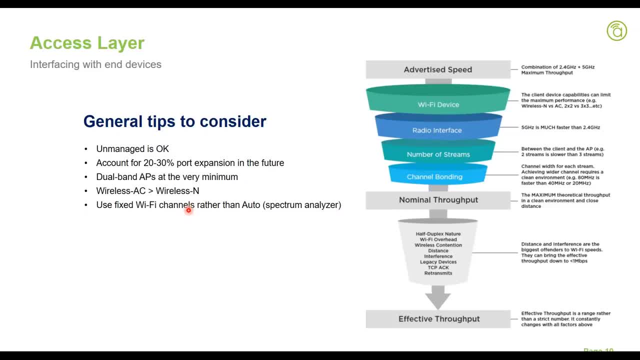 you will pick the right Wi-Fi channel for each radio interface that will have less interference and you know what you're getting into. you will not rely on any external factors for that. and if you know, six months from the from the fact the customer calls you say hey, my Wi-Fi slowing down, you can quickly do another. 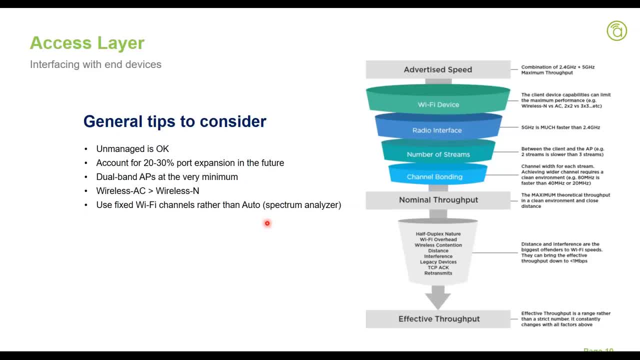 Wi-Fi spectrum analysis and see what happened to that channel and you can jump on a different channel heat map for fine-tuning- and this is when your investment in heat mapping software will be very important. to set the expectations right, make sure that you don't have any. 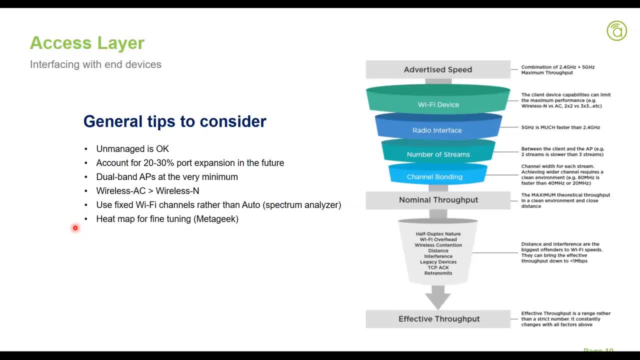 dead spots in the Wi-Fi coverage. make sure you measure the speed. so this, these tools, will measure the speeds, that distance and will get you- you know, you get- a really nice report for your customer to see what the expectations are named interfaces. this is even more important to name interfaces than the. 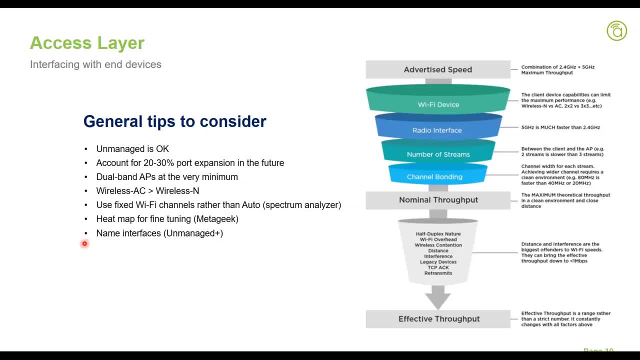 core layer, because this is where you connect your Apple TVs, where you connect your touch panels. so naming the interfaces is very, very important at this layer and this is really the genesis of our 110 unmatched plus solution. this is why we believe our 110 series switches are imperiled in the market, because you can do basic. 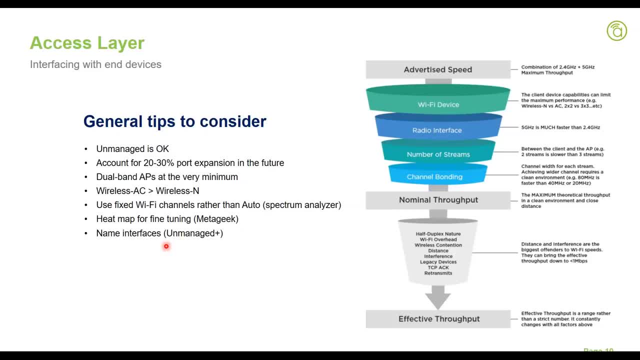 management features through oversee. you can name those interfaces through over city, rather than getting a dumb switch that you cannot name. so this is what. what sets this the 110 series solution, apart from everybody else in the market. very, very, very important is to name the cables and test them. I can't. 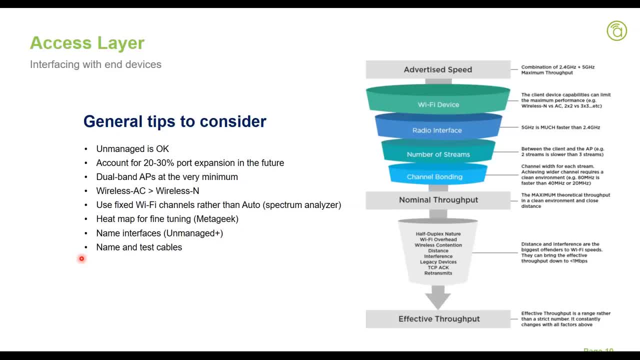 tell you how many times we get calls from dealers thinking that the port is problematic in the switch. it turns out to be the termination is not good or there's something happening in the cable is not tested or is cut off. your cable infrastructure is the backbone that runs everything, so if your cable is good, your 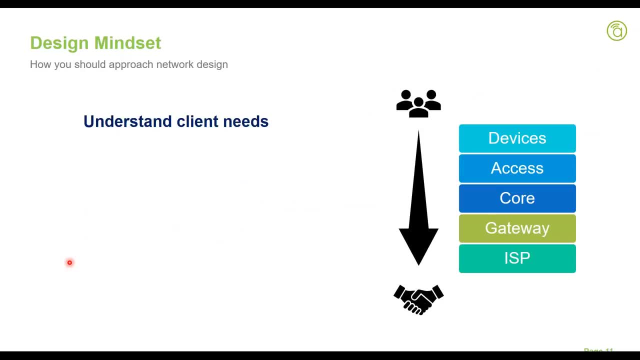 network is good. now we'll shift the conversation over to the next slide, please. We have that framework from a design perspective. when you sit down with your customer and you want to design a solution for them, you you need to flip this model framework upside down, so your conversation with the customer should. 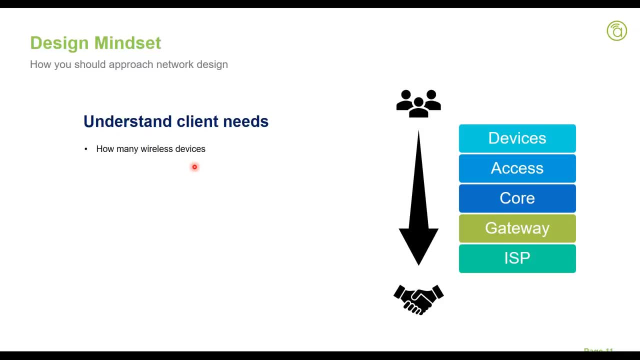 start with the devices and the devices. you should ask like, hey, how many you know? how many you know family, household, or how many members that, how many people that will be at that in that location, how many wireless devices in total and, on average, how many wired devices they will have on average, you will add a lot. 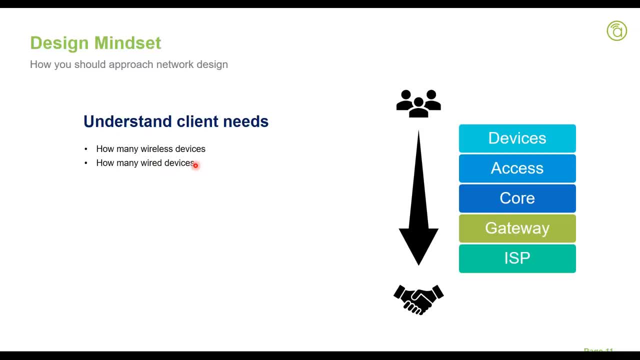 of devices on the network, from other solutions like your AV solution or your thermostats and what-have-you. what services are needed? they want to stream music. they want to do some surveillance. you have some control system, some lighting control. this is. these are the normal steps that you go through with. 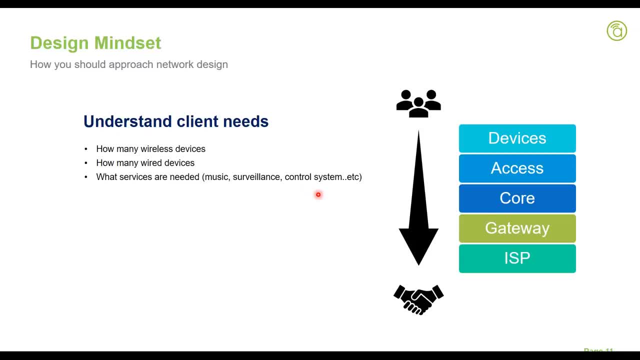 your with your customers, but as you go through them you start to map out in your head what that network architecture should look like you do. I would highly recommend to do a quick site survey of the floor plan and do some initial wireless design to determine how many access points you 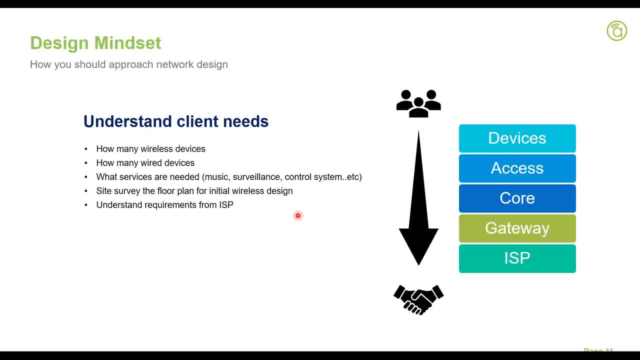 need and when you want, where you want to place them, understand what kind of ISPs are in the region, what kind of bandwidth they want to get from that ISP and then, like I said, the expectation is about the Wi-Fi SPs. based on our webinar, they will 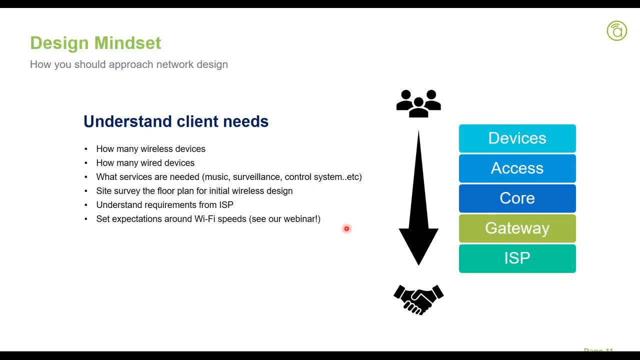 not get. you will never get one gigabit per second Wi-Fi throughout the house. that is not going to happen within the existing standards, no matter what other vendors tell you. explain the higher than the need for higher networks. unfortunately, we still see hear from dealers that there is a pushback around the quote for 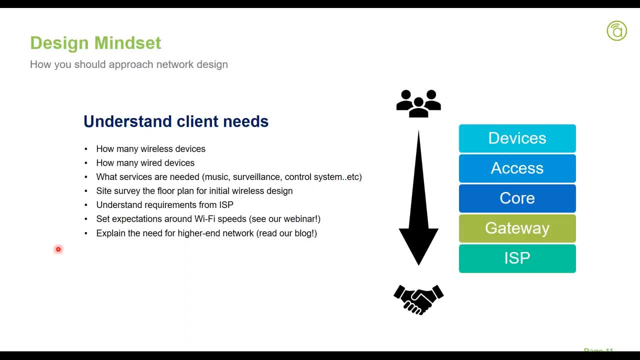 networking in a higher-end job. it is very important for you as you under, as you face these challenges every day, because the network is a very important part of your business, and it's very important for you as you, as you face these challenges every day, because the 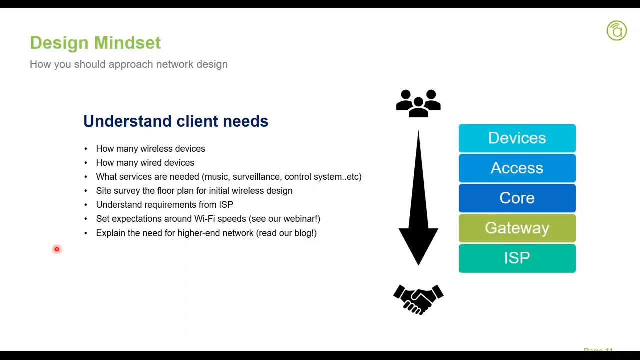 network is a very important part of your business and it's very important for you as you work as the backbone of the solution. if you don't own it and it's not up to speed in terms of performance and reliability, then the end user experience is not going to be as good. then you do your design and you quote it. 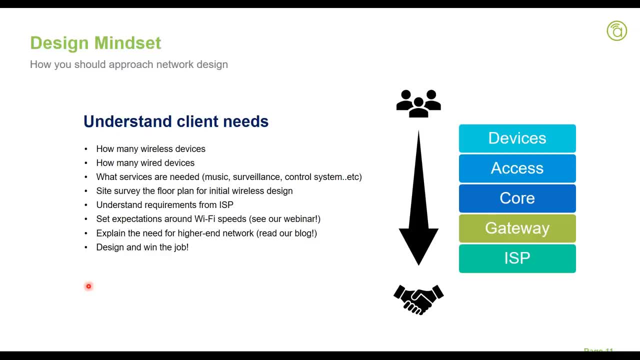 and hopefully, you win the job. so this is what we think, our general steps, or general tips that you need to take into consideration when you sit down with the customer trying to design the job or quote a job for them. now, before we turn into the next slide, 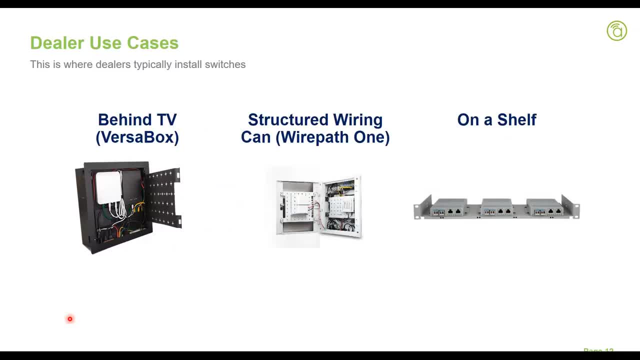 to the Q&A session. we'll get to the product announcement phase of the presentation. we're super excited about the outdoor access point that we launched last week. lots of great feedback, a lot of excitement and we see it in the end- the sales numbers. today I'm gonna announce a product that we 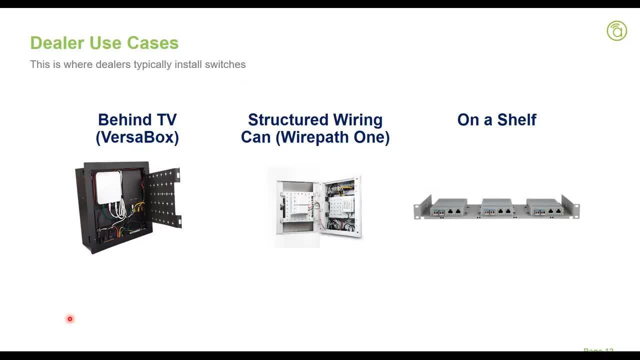 released next week. so when we sat down and thought about those use cases that from a networking architecture perspective, we see, we hear from the dealers that a lot of time they put their switches, especially those access switches, either behind the TV and this one versa box will come into play. 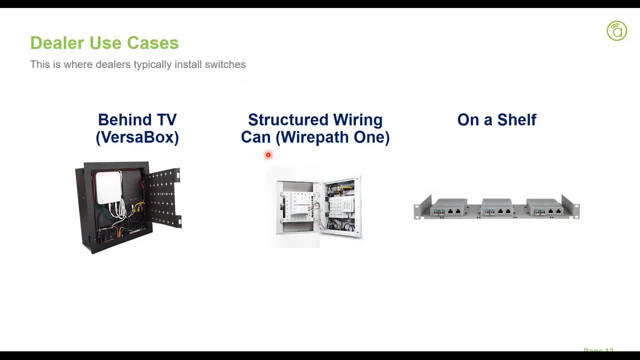 or they will have a structure wiring can in the job and they want just to loop in and out that structure wiring can into the centralized rack, or they put it on the shelf. so they they have, you know, a shelf in the rack and they have an access to a small device like a Roku they would like to keep with another. 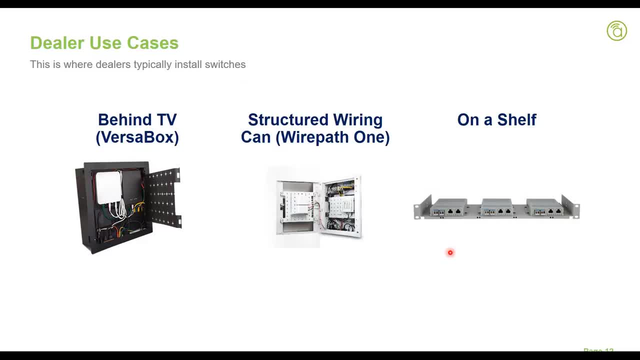 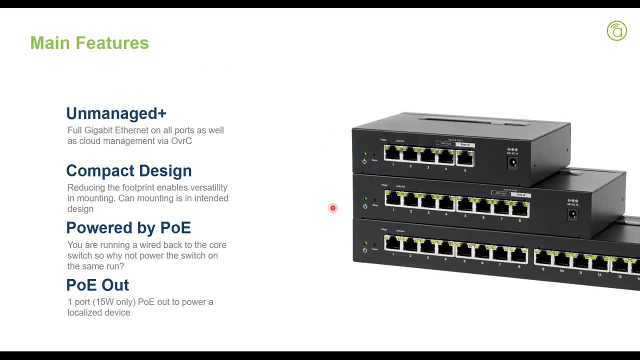 switch right next to it to save some space in the rack. so this is why we developed the new one-tang compact series line. so this is an expansion on the existing 110 series switches. so it comes because it's 110. it's unmatched plus, so it's full gigabit. on the back plane, it's cloud managed through oversee. 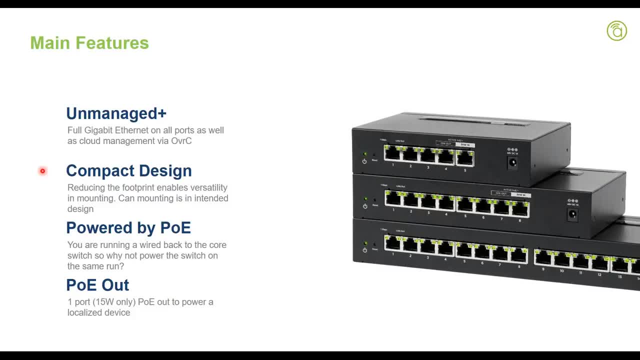 like I said, there's nothing like it in the market. it is very compact in design and I will speak next on on what are the benefits for that compact design. they are powered by PoE, so that's very exciting from an architecture perspective when you have a core switch that is a PoE and you have a TV location. 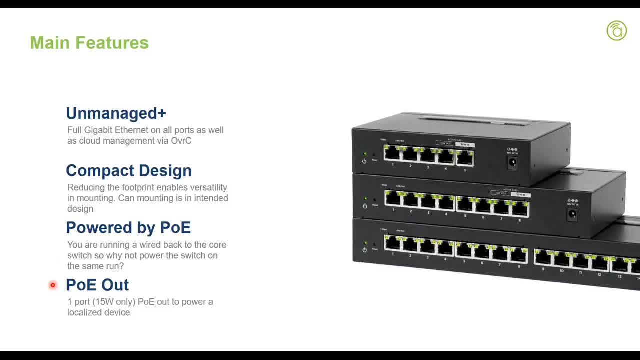 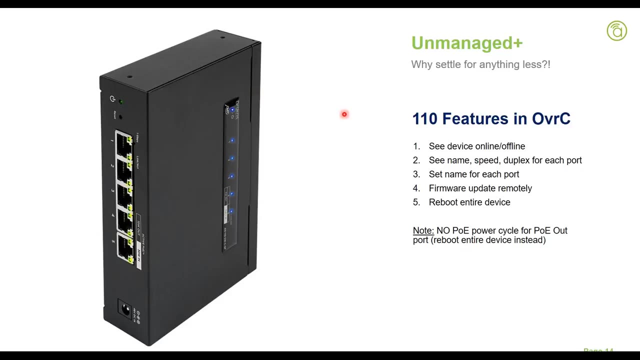 and you want to put a five port that is powered by PoE and there is a PoE out. so, whether it's powered by DC or powered by PoE, the PoE out is 15 watts. so let's go quickly through the feature. so on managed plus. like I said, it's an unmanaged switch, but cloud managed. 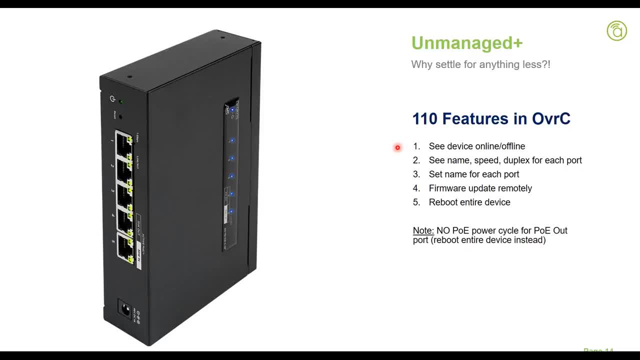 through oversee. so it's DHCP out of the box. it grabs an IP, talks to oversee. what do you get in an unmanaged switch? is you see devices online, offline? you can see the switches of offline or online. you can name the switch. you can name individual ports and you can see the speed and duplex on each port. you 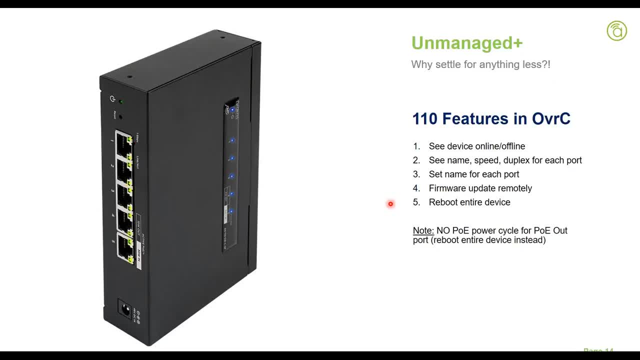 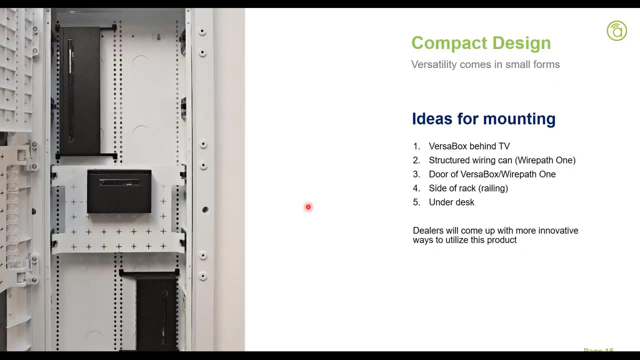 can do firmer updates remotely, if we do any firmer releases and you can reboot the entire switch remotely. so we cannot- we couldn't get to reboot the individual POE out, but you can reboot the entire switch and that by default reboots the POE. so, like I said, 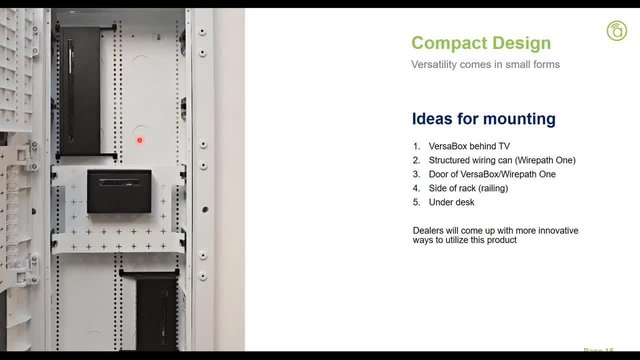 the compact design. it's very, very important. so we went into this product design from the mindset of let's design a product to go into a structural wiring can or or into versa box so you can see it comes in five, eight or sixteen port option. they come with the mounting gear included in the box. there's no DC power. 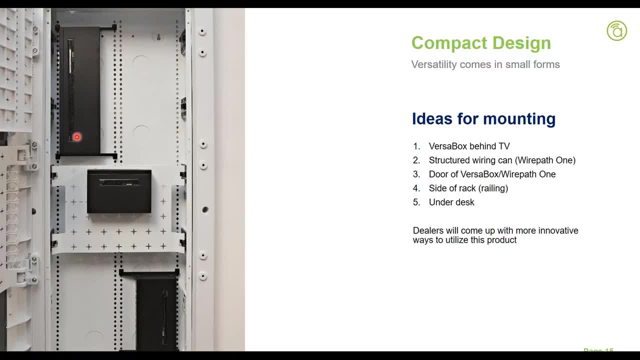 supply. but you can see it mounts very neatly, very nicely into the structural wiring can and you can put it here. if you use our wire path, one cans, you can mount it on the platform. we've seen dealers and during beta tests that they do mounting on the side of the rack sometimes and they do it under the desk. 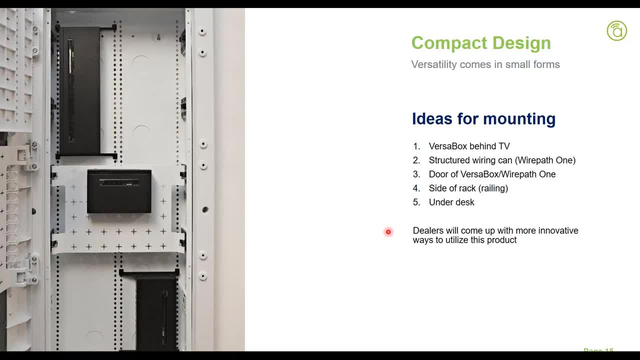 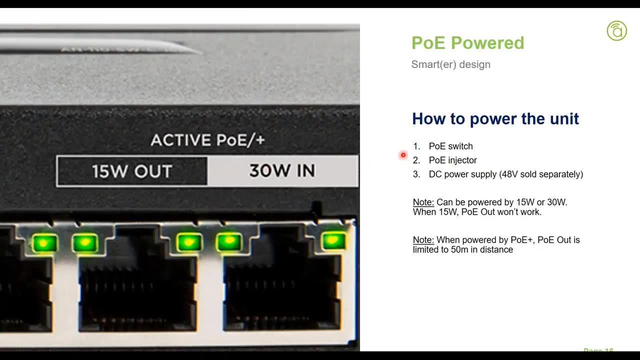 and I'm pretty sure you guys find a lot of innovative ways to install this product. Like I said, it's POE in, so it's 30 watts in and there's 15 watts out. it can be powered by either POE switch or POE injector or a DC power supply, the DC 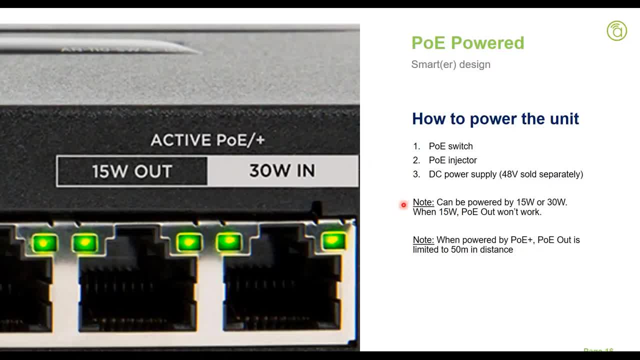 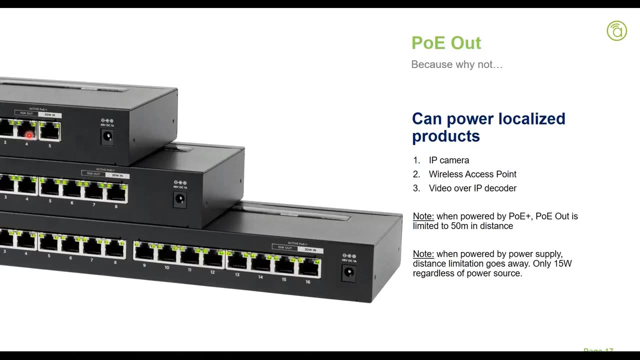 power supply is sold separately. it's 48 volt, but when you power through 15 or 30 watts, it's it's 15 watts only POE out. so you can power another localized device like an IP camera or a wireless access point, or you can power actually another compact switch. 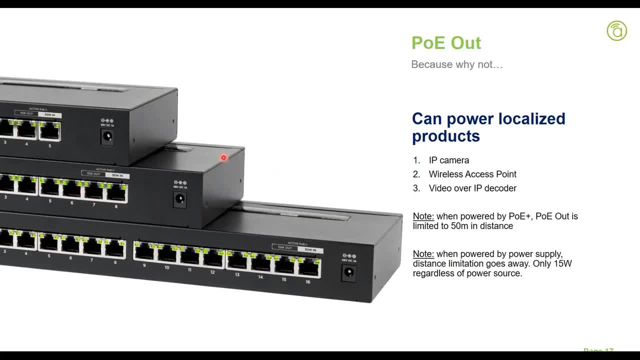 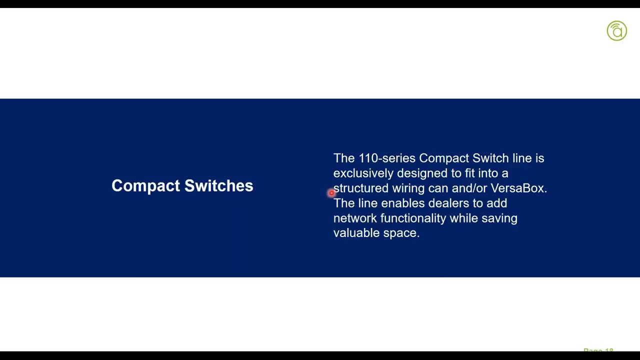 from another switch by POE, but be aware that the POE out, when powered by POE, is limited to 50 meters. in terms of distance, that's about 150 feet. so that's it. that's the announcement. it's compact series. that's really our design process. 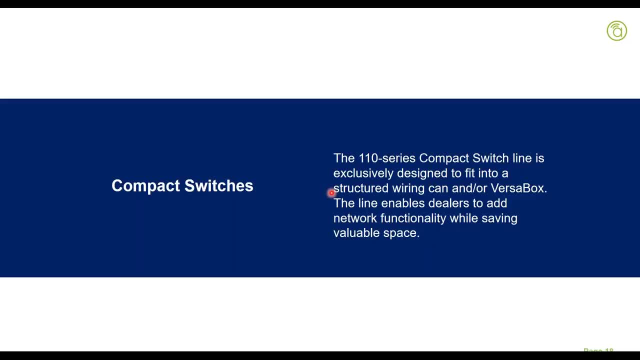 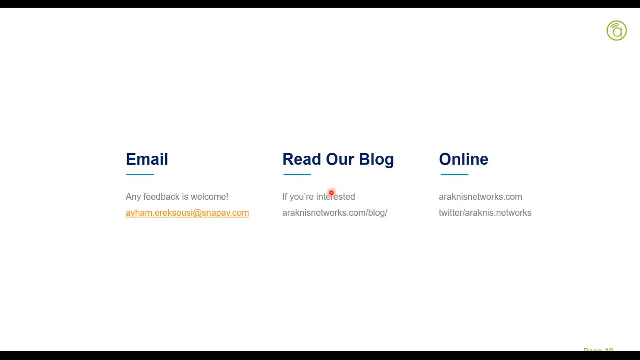 to go into the custom installation, listen to your pain point and design a product around those pain points and give you a really valuable solution. and, with that being said, I'll leave it to Ricky so we can go through some questions. All righty, Aham, as always, great information on networking. we're gonna go. 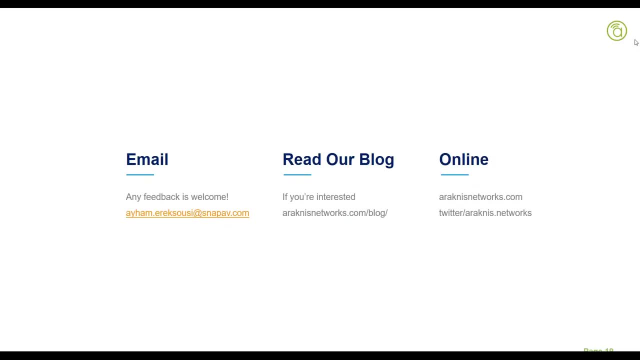 through a few questions here. I think most of these everyone could get a little bit of good answers on. some of these. most of these we did cover, but I think some of them are pretty important that we would maybe cover again. I saw this last one. we just talked about the POE. 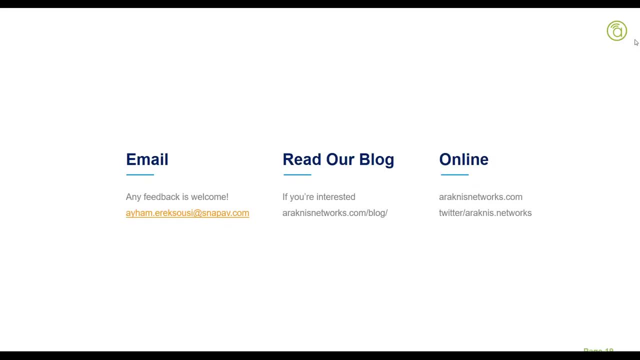 capabilities of these compact switches and one of the questions, The Hия, is: is this POE plus device or will it only pull 14.5 watts? so I think you cover that, but once you go in a little bit more on that, that's a good question. so it is both. it depends really. so the switch itself it. 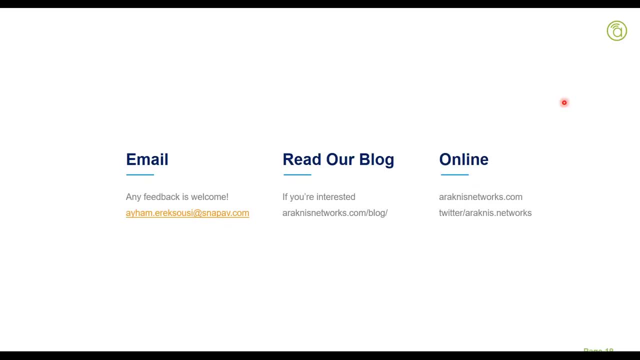 pulls up to 12 watts of power. but when you power, when you utilize the POE out. so if you, if you're not utilizing the PoE out interface, then it's only PoE. if you start to pull power from, that PoE out interface now becomes a PoE plus n. so 30 watts and 12 watts consumed in. 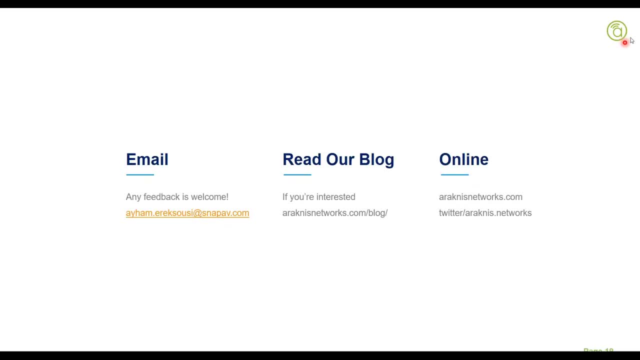 the device and 15 watts out, if that makes sense. okay, let's go into some general questions here and a lot of these. you actually answered some of these, but again I want to reiterate some of these questions. I think they're they're key for the networking guys. do you need a core switch if you only have one access switch? great question. no, in that case, when you have a really small job, and really small means that you can have up to 48 devices on a one switch that can act as a core and access switch, and you can have up to 48 devices on a one switch that can act as a core and access. 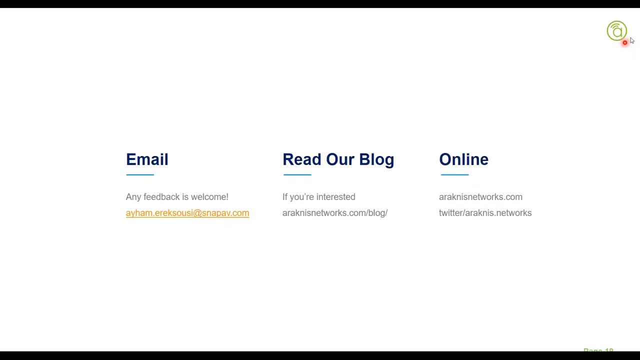 switches at the same time. you do not need a core switch. this is really more of an expandable and scalable architecture when you have those larger jobs. but let's say I have a small to medium-sized job that I got you know- up to 48 devices only. they need no V landing or they need it just to. 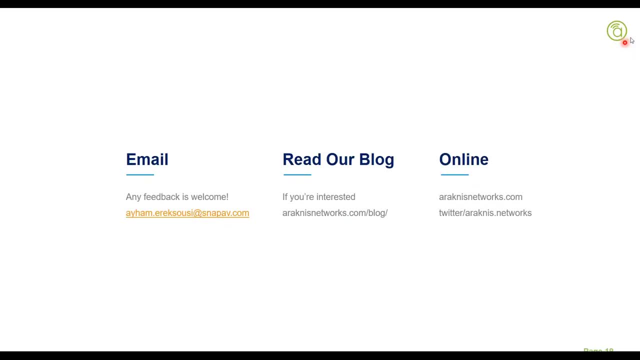 be plugged into one device. then you can get a router and from the router to a 48 port switch and then from the 48 port switches all the way to end devices. that's very feasible. okay, you may have to pull up one of your other slides for this one, but I think it's key, please. 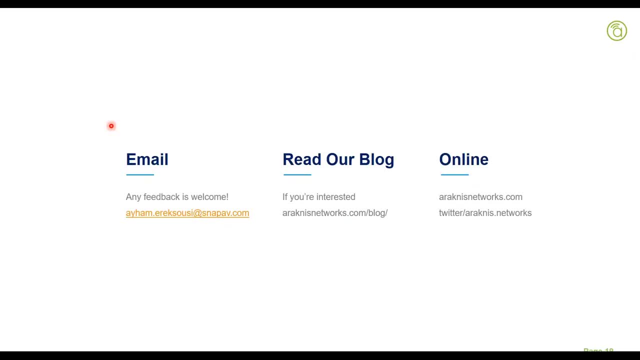 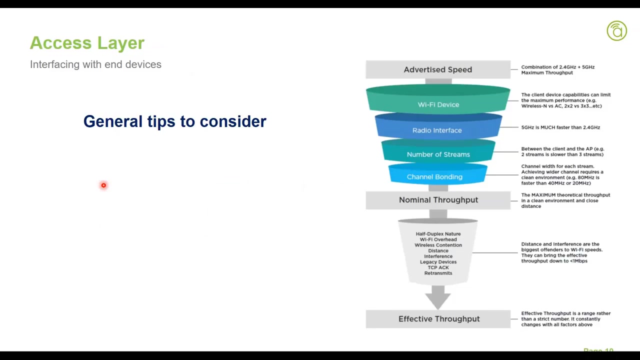 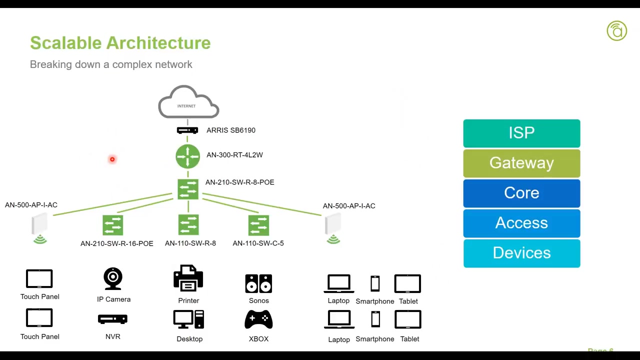 discuss the location of the oversea hub and why you'd put: oh, great question, great, great question. let me go back to my architecture. one real quick up, here you go. so great question, your oversea hub, since it's measuring speed and latency, ideally what you want. 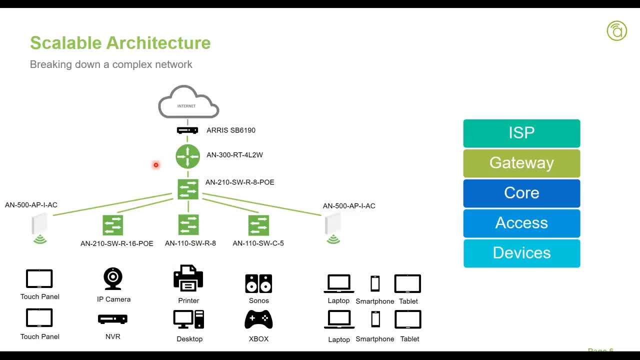 to do is plug that oversea hub directly into the router. this is the best place to put the hub because it will go only one hop to the internet and also it will be on the top of the network to scan the entire network. we are so today. if you put today the 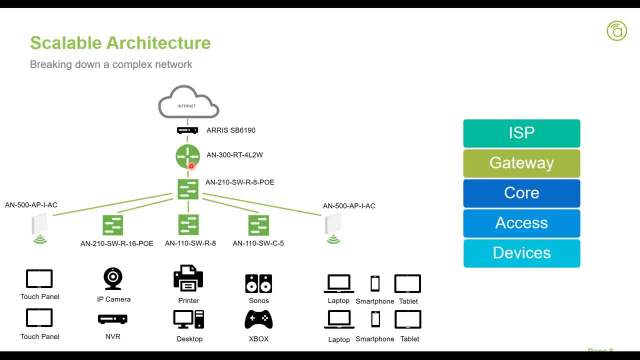 up to the router- our existing 300 series router- you will see there's a significant dip into the reported speed and that's a bug that we are fixing in a firmware update for the router that will be scheduled to be released by the end of the month. so in a couple of weeks we will release a new. 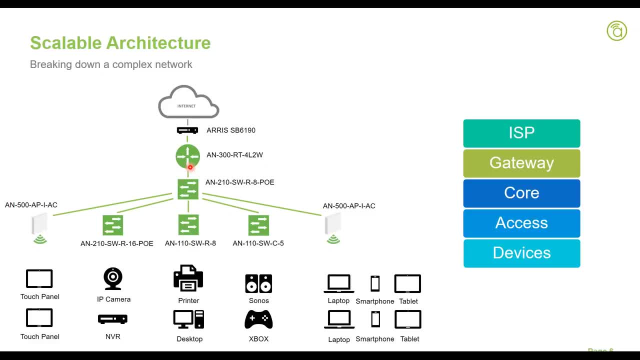 firmware for the router. it's 1.0.5.34 and that will fix that issue and you'll put the hub. your next best option today is to put the hub into the core switch again. you want to have as accurate of speed as a measurement as possible and you want to have as as good of access to the entire network as possible. 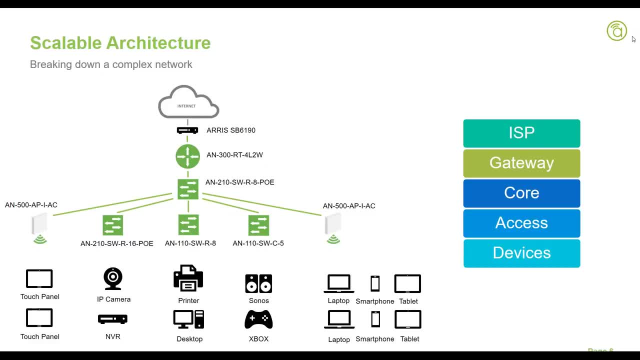 so that's a good question. okay, again, I think we covered some of this, but I just want to make sure that everyone understands. if there are only two switches on a network, are you saying we should have the layers stacked, one off the router and the other off the other side? so that's a good question. so that's a good question. 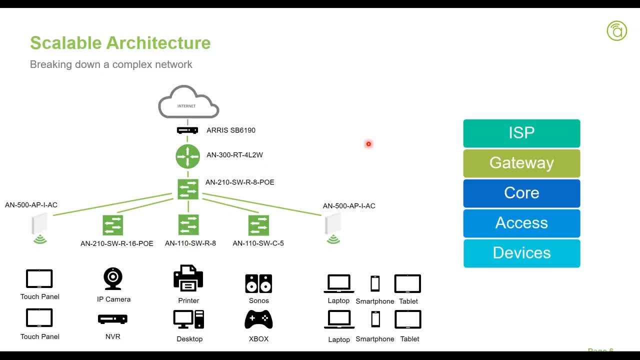 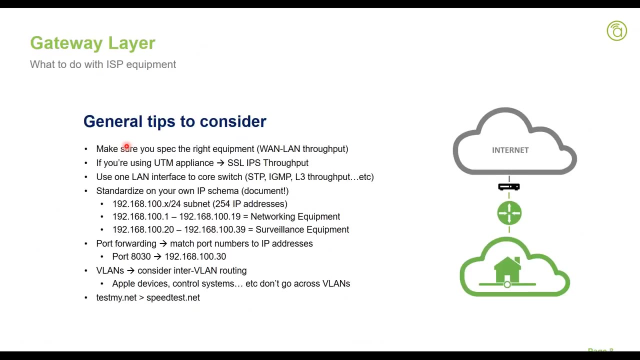 it depends on on your architecture, but ideally, yes, you do not want to have two switches off the router because you, like I said, you will end up with a situation, uh, where you have- let me go to this slide- when you have traffic going, if you have traffic going between those two switches. 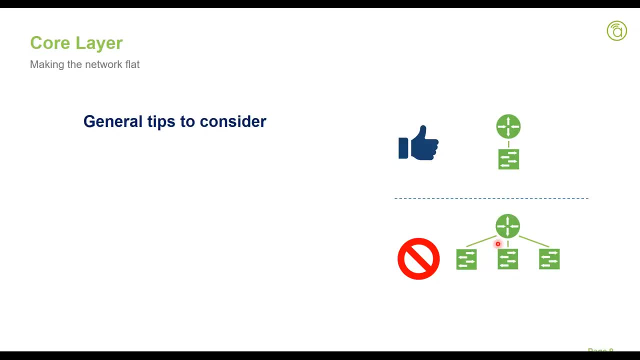 they will go through the router and now you will have spanning tree issues, you will have IGMP issues, um, if you have any inter-vlan routing between the two, you will have performance degradation for sure. so ideally you want them to be one off the other one as a core, one as the axis. 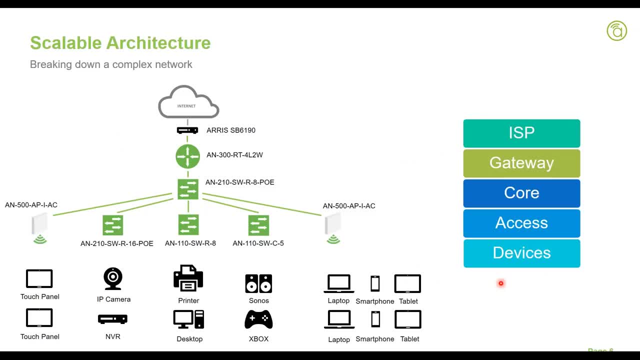 all right. so again, lots of questions about that. so just everyone. so everyone's clear- is that there should be one core switch and then other switches plugged into the core switch. so when you're designing your system- that's why it's so important to understand how many. 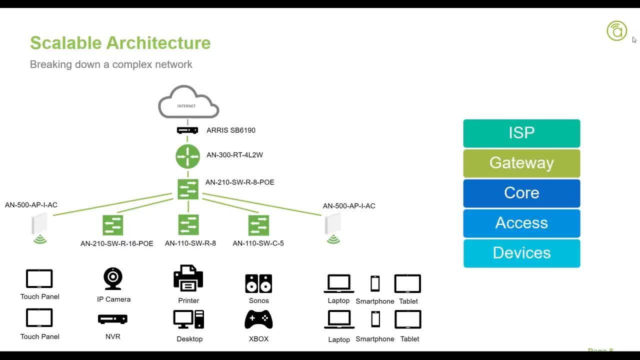 network connections you need to have, uh, to how many devices? so another quick question here. uh, this is just a general question: what IP finder tool do you recommend for Windows computer? any recommendations on that? um, good questions. so we got a you know, a couple of options. uh, some of. 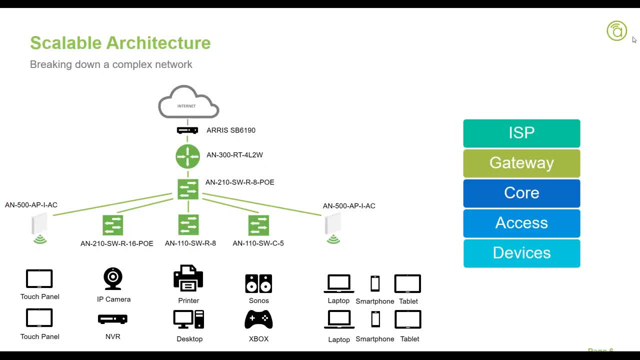 them are free. so if you are using uh Wi-Fi, uh on the phone- I'm a big fan of thing- um, I think is a tool if you are using, obviously, our oversee help. oversee hub utilizes multiple tools inside the code to sniff the entire network and puts everything. 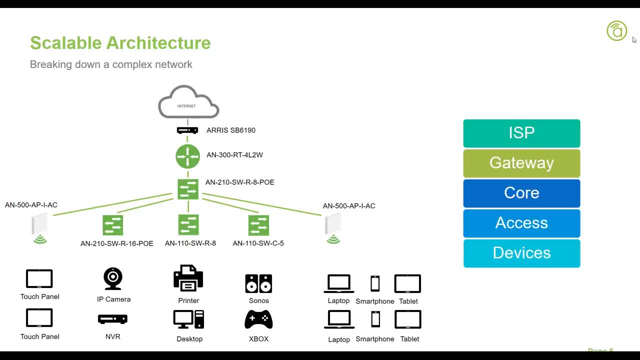 into your oversee dashboard. if you just wanted something that is software on the PC, I think for Windows there's a Windows IP scanner, if I if I recall that correctly. all right, just a couple more questions real quick. this one's on the compact switch: how small of these? and do they need any airspace? they're quite. 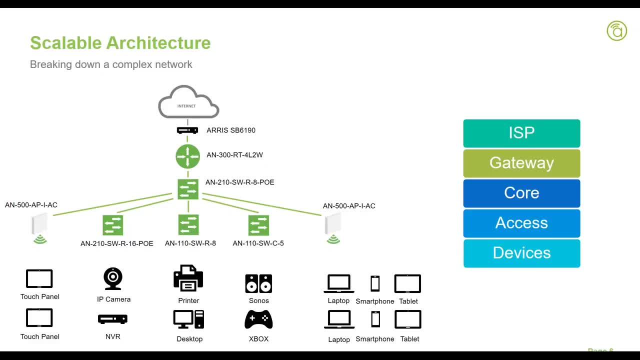 small so you can see them. they are on the website. that's coming soon items. just filter on the left side, unmanaged plus and you'll see them as coming soon. they're quite compact. you need some airspace going. just because they are fanless, they don't have any fans, so you need 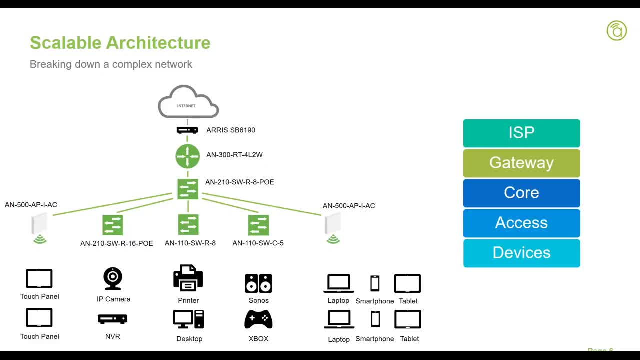 some ventilation going through the switch. but like, for example, we we during the design process, we we thought that would be a good idea to do a drop-in installation in the versa box similar to the WAP box. but unfortunately that tight space is not recommended by the certification bodies because of 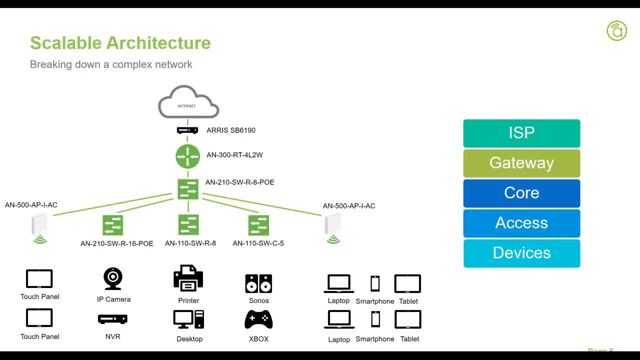 you know air circulation, the risk of running too hot and and catching fire, so that you do not want that to happen. so make sure there's a good amount of space around them and for all righty. another quick question: can you talk a little bit about the proper 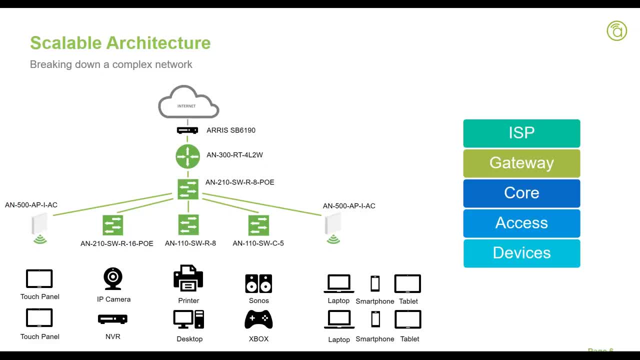 use of the SFP ports every like if you have 10 long Laser for quite multiple use cases, the full time restoration. can you hear me now? sorry, I lost my connection for some reason. so there's FB port, so two, 10 and three tenths, which is that we have. there are. 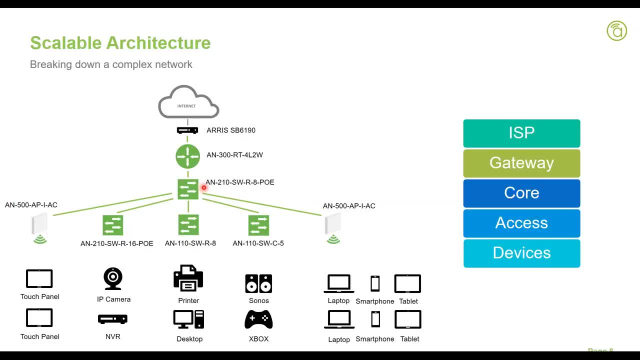 at minimum two SFB ports and a maximum for SFB ports that we, any port that we. when you have 48 port models, so those SFP ports, they are extra ports on the switch. they do not share any backplane with other ports, so they have dedicated. 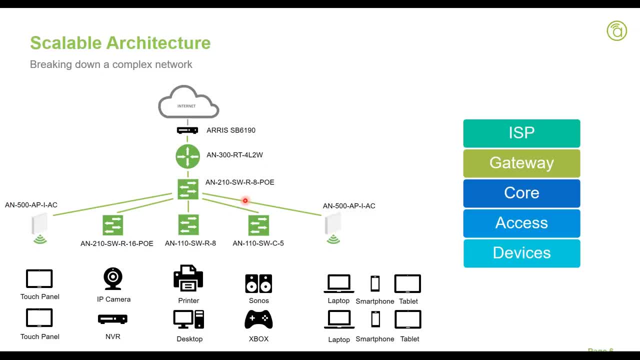 bandwidth. so really an 8 port is a 10 port. but when it comes to SFP ports, there are really two use cases that we recommend that we see dealers use that for. so the SFP port, think about as an empty slot that you can populate with. 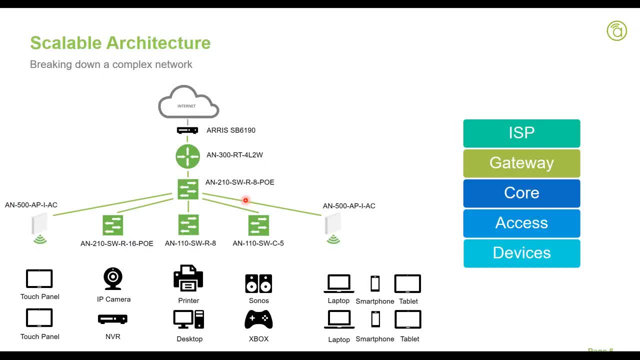 either electrical RG 45 or a fiber SFP. so let's talk about the electrical RG 45, if you have. let's take this example: we have a job. when we got, you know, a 210, 16 POE and 15 or 16 of those POE interfaces need to power 16 IP cameras. you still 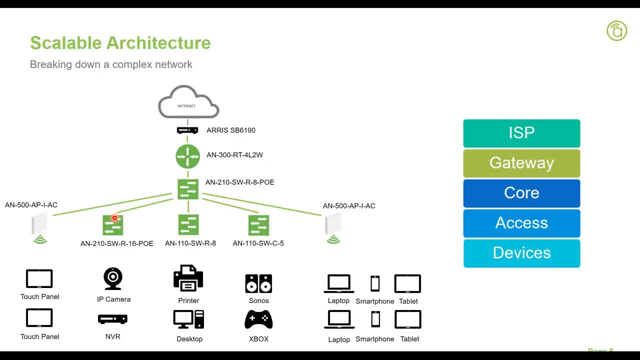 need the one interface to go back to the core switch, so that interface is the one interface that you need to power 16 IP cameras. you still need the one interface to go back to the core switch. so that interface. it's easy. you have two option: either you lose a POE port or you get a RG 45 SFP. 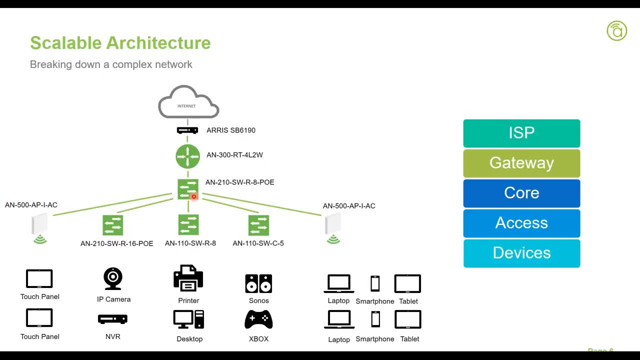 and plug that RG 545 SFP and connect it to the core switch, and now you have 16 POE ports going to 16 IP cameras. because so that's a main use case. the other use case is think about, for example, this 5 port or this, you know, instead of the 5, 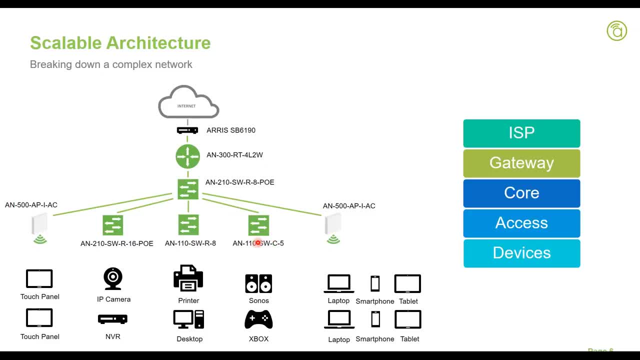 port here there's a you know 8 port 210 and it is in a a a a guest house, but is really far. it's like 200 meters far, 300 meters far. your RG cat 5 from an Ethernet perspective can go up to 100 meter tops per. 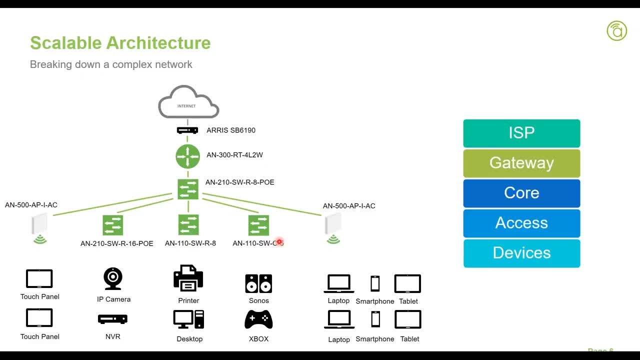 standard. so that is 350 feet. if you want to go beyond that you need to go fiber. so if you will have to go fiber interface, then you would populate a fiber interface on the switch in the access switch and a fiber interface on the core switch and now you have the fiber link between the two switches. 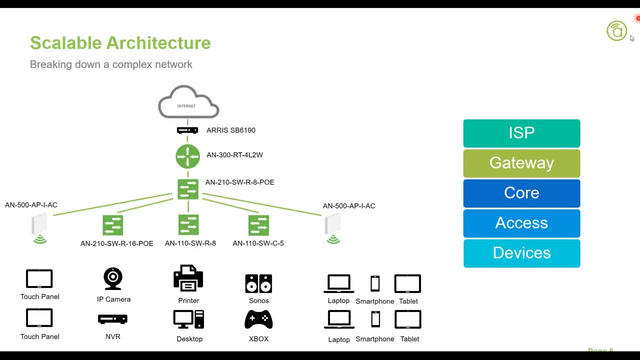 all right, we're about to run out of time here. I got one more question here. I think it's pretty relevant. we didn't talk a lot about the brand new outdoor wireless access point, so this question could come into play here also. by the way, on the on. 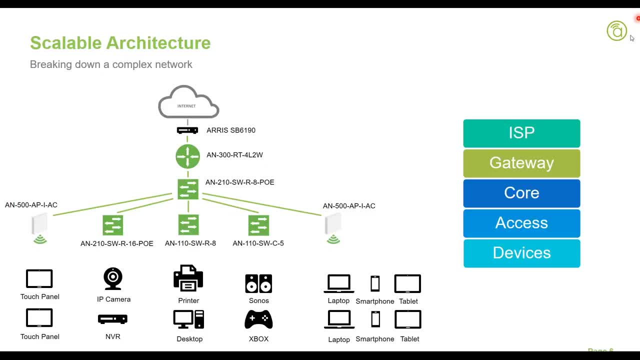 the wireless access, the new outdoor wireless access point. there's some really good videos on that product tab that you might want to take a look at, but this question just came in: can I just add your new outdoor wireless access point to a customer's existing network? so I think a him you should. 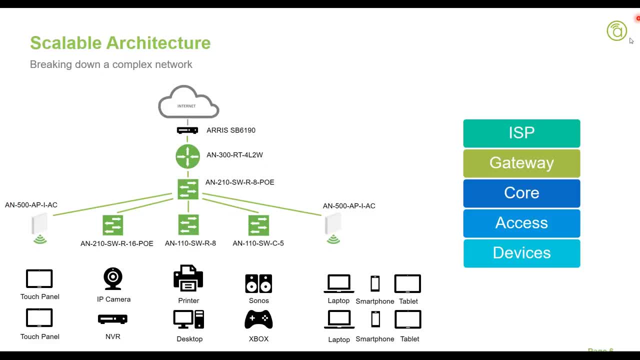 probably talk a bit about the power requirements and things for that. yeah, the quick answer is yes from from for the outdoor access point 700 series outdoor access point. it has almost the same software features as the indoor 700 series outdoor access point. it means that you get dual band, concurrent 2.4 and. 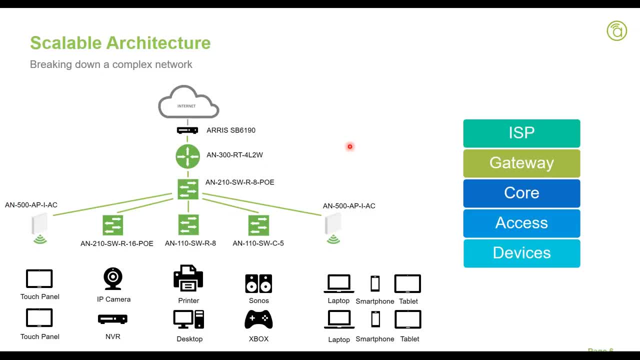 5 you get 1750 wireless AC with 3 by 3 and antenna and in that support tab video we talked about, you know it has the same band steering, it has the same fast roaming features, so it will work seamlessly. it's overseeing enabled. the one caveat, or the one thing that we did. 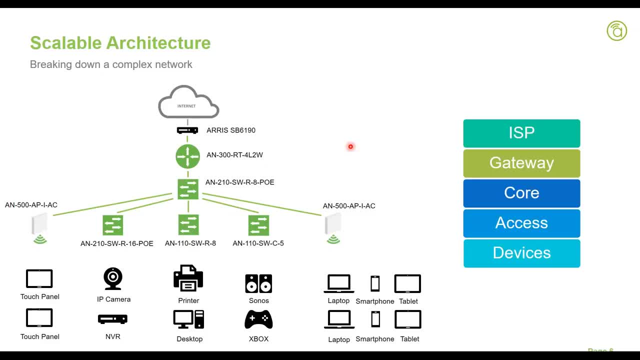 from a design perspective and it's because it's an outdoor product. outdoors, in the outdoors, signal travel really far because there's less obstruction, there's less interference, or not. there's more interference but less obstruction, so it doesn't degrade that much. so what we found in testing is that you know you will be sitting 400 to 500 feet away from 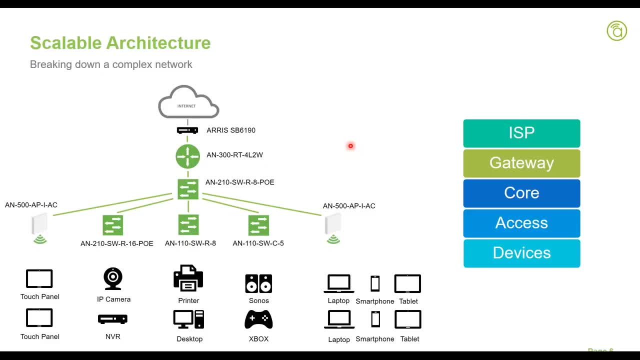 the access point. your phone will get two bars of Wi-Fi coverage, sometimes three bars because it travels really far from the access point. but your phone or your tablet is limited in its output power, or so think about it. that's its mini access point. there's a radio inside that phone that needs to transmit. 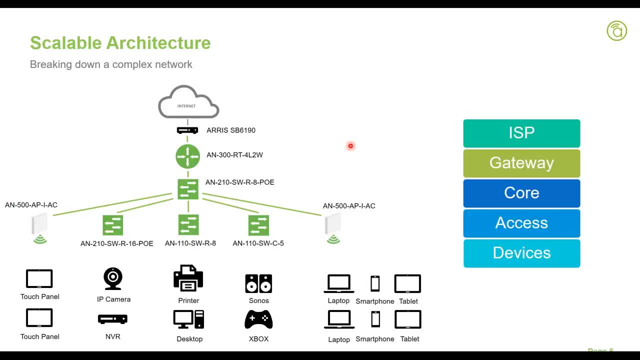 power. so the maximum power for that phone is 22 dBm. and when you have a really high powered access point, that reaching really far, and that signal strength coming from the phone back to the access point is not as high, then you end up with two bars of Wi-Fi but you're spinning because your signal you cannot. 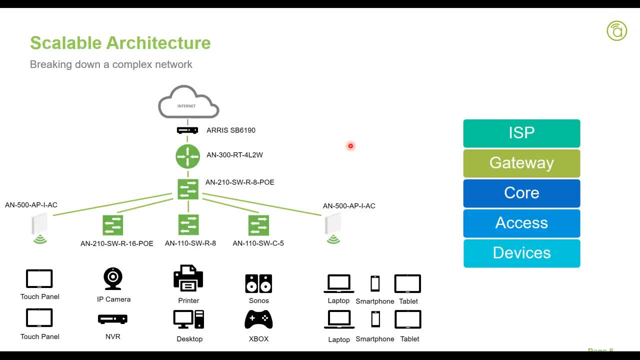 talk back to the access point. so what we've done with the outdoor is that we need two bars of Wi-Fi that are connected to a motor and two bars of Wi-Fi that are connected to that device, and that we're testing this out and I've been using 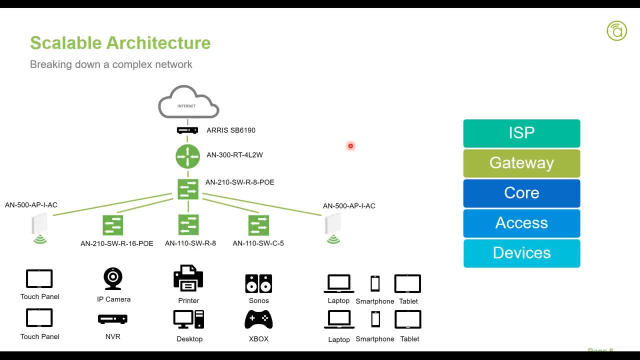 this for a while, but it's just not working as good as it used to, or it's not like it worked, or something. so I've been using this for a long time now, so you can use the Wi-Fi up in a lot of other places, or you can use it and then. 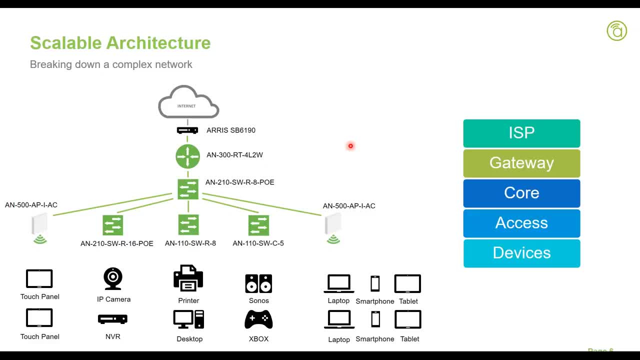 it's very much the same. we don't use a lot of power. the Wi-Fi does that. you can use a lot of power, but there aren't many devices that do that. so the thing that I was just saying is that it's very similar. you can use this to get a. 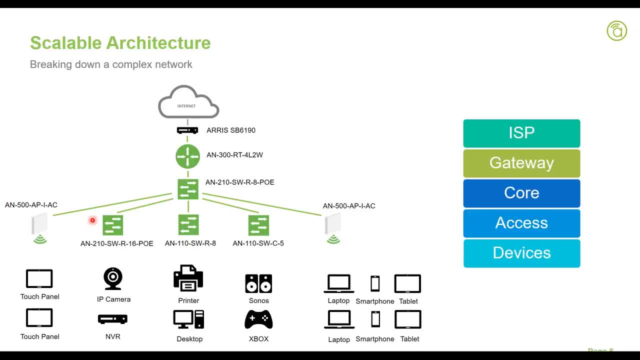 but from an installability perspective and from an architecture perspective, it's really plug and play. It will be another access device on your access layer. All righty, That's about as much time as we have for today. There are quite a few other questions that have come in. 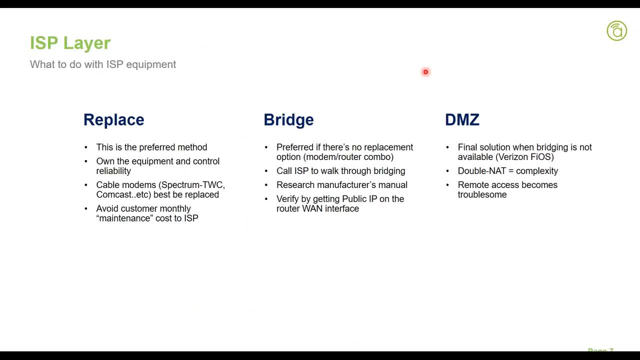 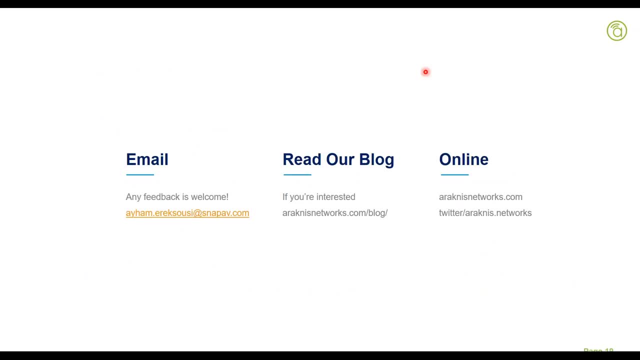 And, of course, like always, we'll pass this on to Aham's group And those guys usually follow up within a day or two on answering any questions that we didn't have time to cover. I do want to add one little bit of information, a personal part of information, to this. 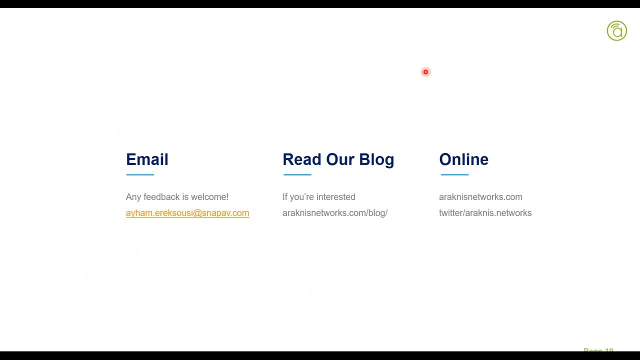 is that every time I sit in one of these webinars and host these for Aham, I learn tons and tons of things that I did not know about networking. I'm sure the same is with you guys. I do want to give you one other bit of advice is that we did a previous webinar called 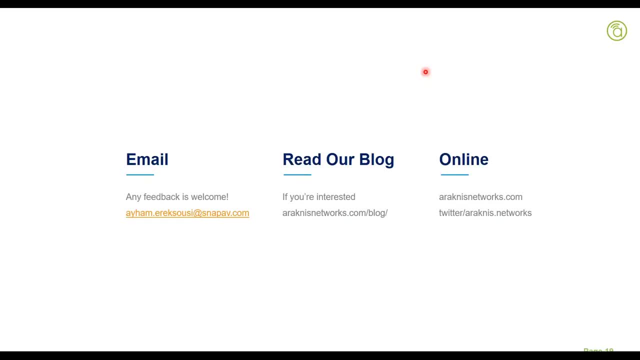 The Truth About Wi-Fi Speeds- And probably it is my most requested link that I get via email- is guys say, Hey man, I want to look at that thing again. Could you send me the link? So I've got to give you guys this advice. 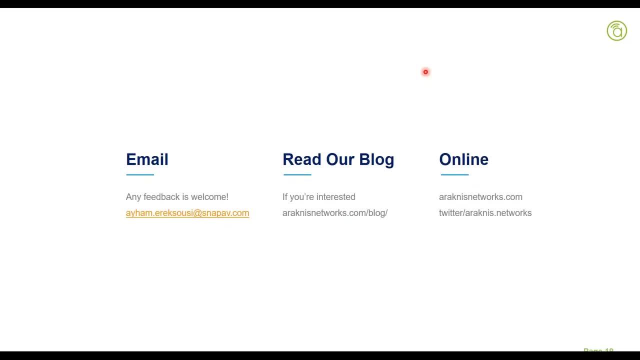 Go to our website, Go to our product pages, Log in with your username and ID, Go to any of the access points- any of our access points- and you'll see a video under the support tab, called The Truth About Wi-Fi Speeds. 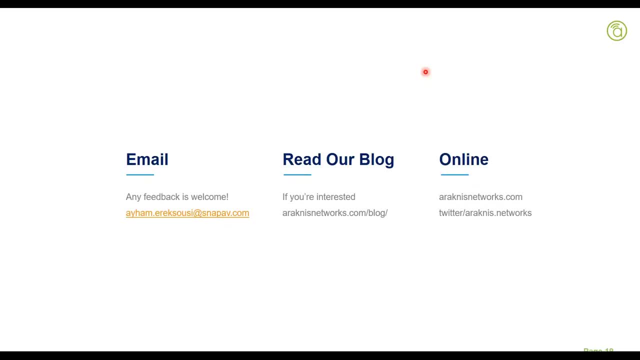 And Aham did an excellent job of being able to explain exactly what you can expect with Wi-Fi technology. I think if you take that webinar, you'll be able to speak, You'll be able to talk to your customers in a really easy to understand way to explain to that customer.